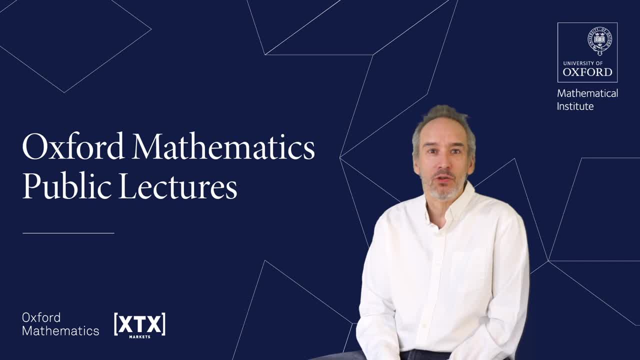 XCX Market are a leading quantitative-driven electronic market maker, with offices in London, Singapore and New York. Their ongoing support is crucial in creating quality content. There has been a lot of talk in the last two months about modelling related to the ongoing pandemic crisis. 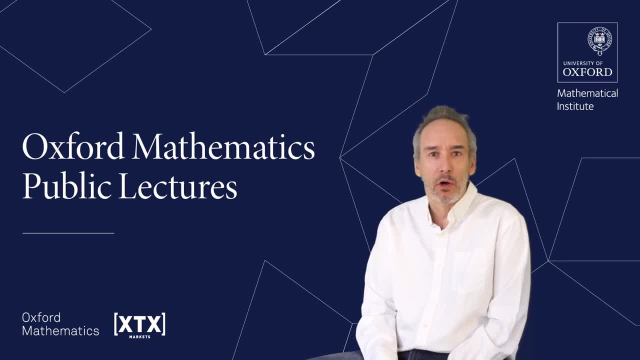 I have found that there is a lot of misunderstanding of what modelling is all about, and we thought it would be important to take a couple of steps back and give you a very broad overview of mathematical modelling in the context of biologics. What does it mean to model in biology, where so much is known and so little is understood? 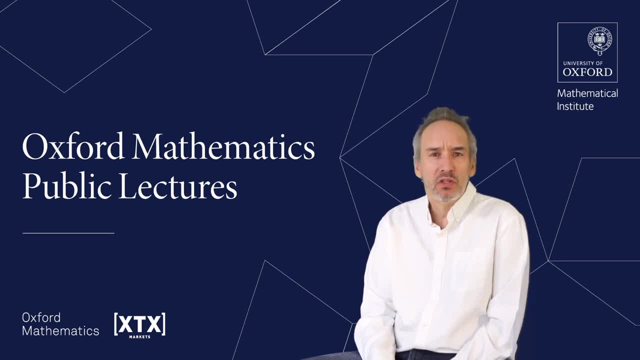 Is the function of a model just to make predictions or to understand processes that we cannot observe directly, or both? To discuss these ideas, I have invited one of the most distinguished experts on the subject in the world, my colleague and friend, Professor Philip Mayne. 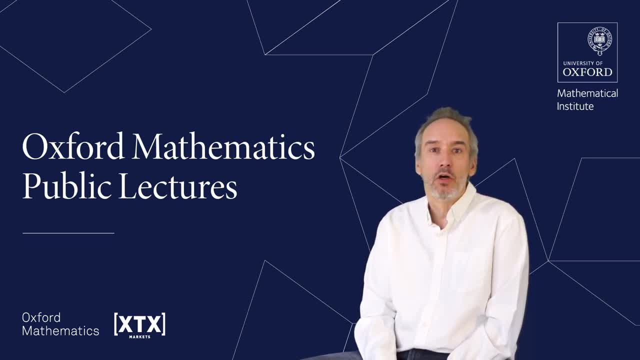 Philip holds the Professorship of Mathematical Biology at Oxford and is a fellow at St John's College. He has made countless contributions to both biology and medicine Within the UK. he has also played a very significant role in fostering a strong school of mathematical biology. 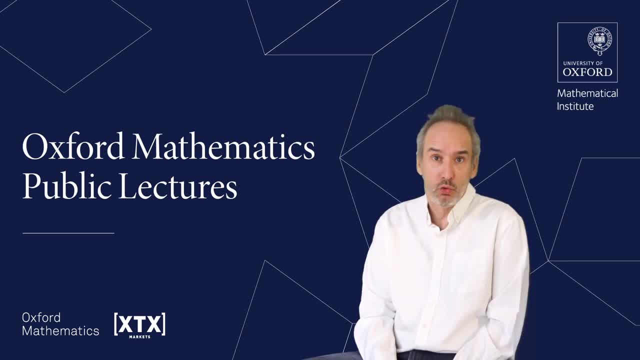 where he has been a wonderful leader and a mentor to many young students and researchers. The breadth of Professor Mayne's contribution is truly remarkable, spanning developmental biology, systems biology, host-pathogen interaction, cancer biology, multi-scale modelling, morphogenesis and pattern formation. 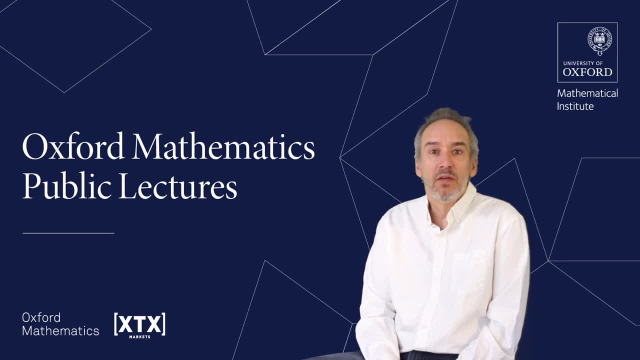 among many others, to both biology and medicine. Within the UK he has also played a very significant role in fostering a strong school of mathematical biology where he has been a wonderful leader and a mentor to many young students and researchers- many others For his contribution. he has received too many prizes to list tonight, but maybe the best. 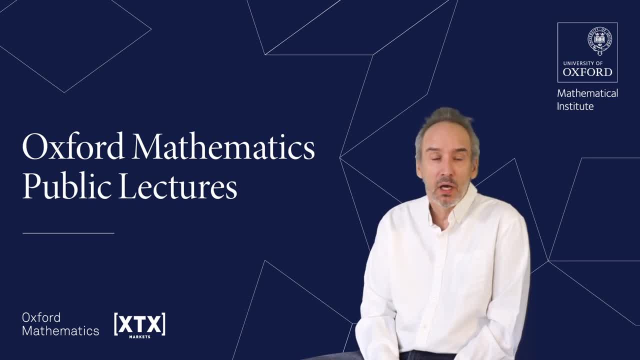 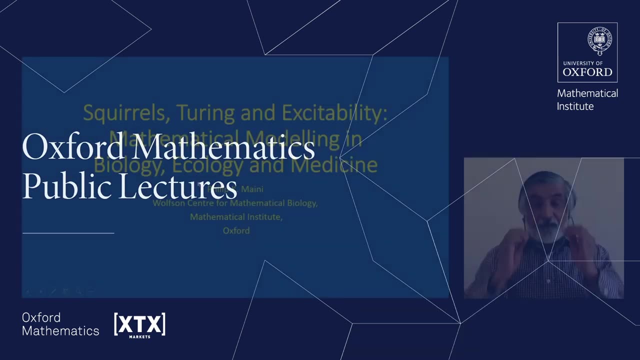 indicator of his multidisciplinary work is his election as a fellow to both the Academy of Medical Sciences and the Royal Society. Finally, I want to add that Philip is also a wonderful lecturer, and I'm very keen to hear him tonight. Please start now, Philip. I'd like to begin by 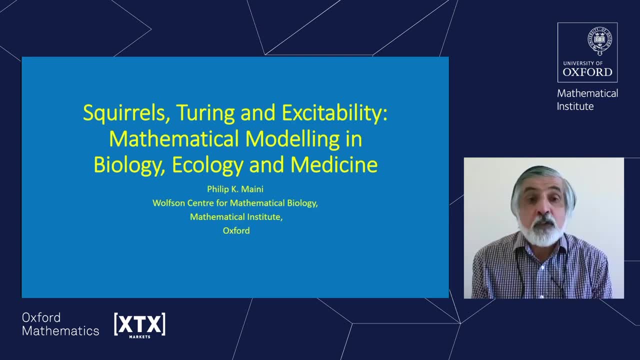 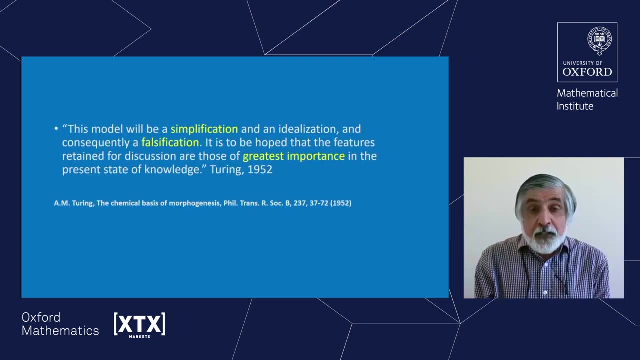 thanking Alain for inviting me to give this talk. I'm going to talk about mathematical modelling in biology, ecology and medicine. So an actual first question to ask is: what is a model? and the best definition I've seen is that by Alan Turing who, talking about his model in 1952, 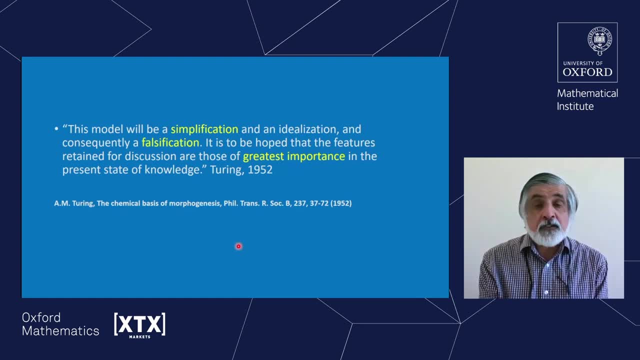 said, this model will be a simplification and an idealisation and, consequentially, a falsification. It is to be hoped that the features retained for discussion are those of greatest importance in the present state of knowledge. So let's see exactly what he's saying. 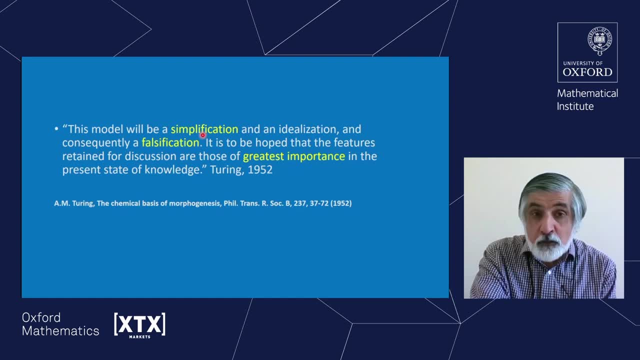 here, First sentence, model will be a simplification and therefore a falsification. That means the model is wrong. because you're trying to understand some complex system, You simplify it, which means you throw things out and therefore, by definition, it's wrong. It is to be hoped So. 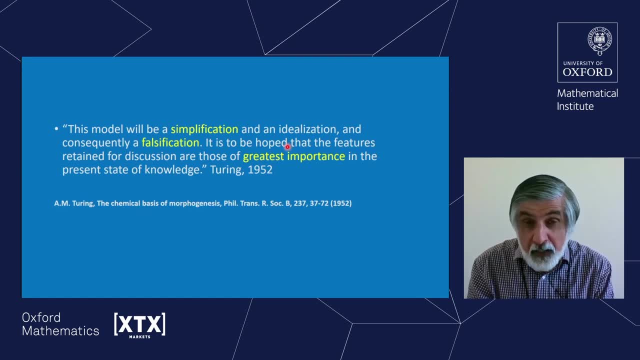 that means that modelling is not a science, it's an art, That the features retained for discussion are those of greatest importance in the present state of knowledge. So if you're working in some medical area or some biological area, the present state of knowledge- you probably don't. 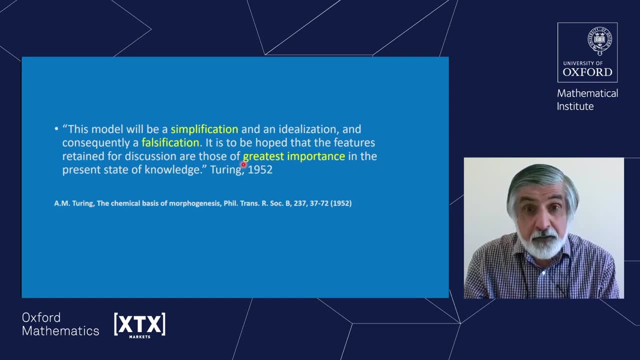 know that. So you're probably going to have to work with a collaborator. The role of modelling is to advance the present state of knowledge in the application domain. So if you advance the state of knowledge, then you might have to re-evaluate your model and start. 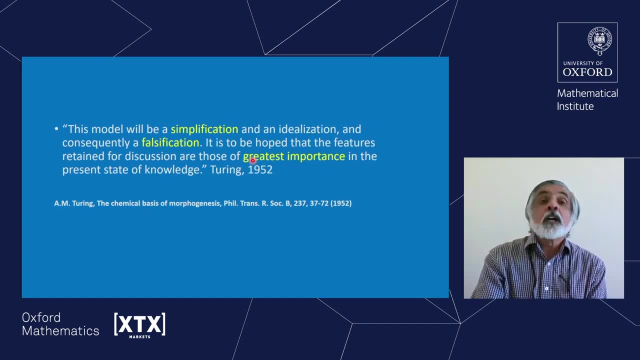 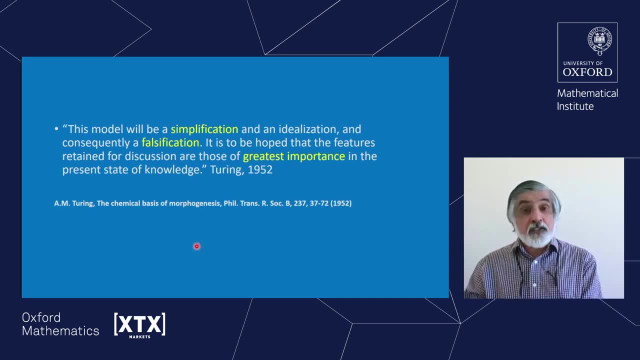 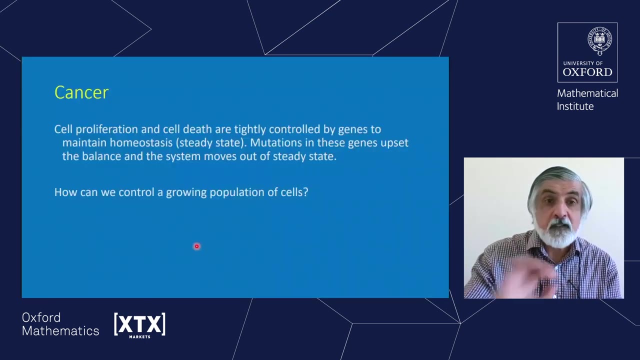 One can draw analogies between many different areas in science and transfer knowledge from one area of science to another area of science. So I'm going to begin by talking about ecology and medicine. So cancer, So roughly speaking, in our body, every day, lots of cells die. 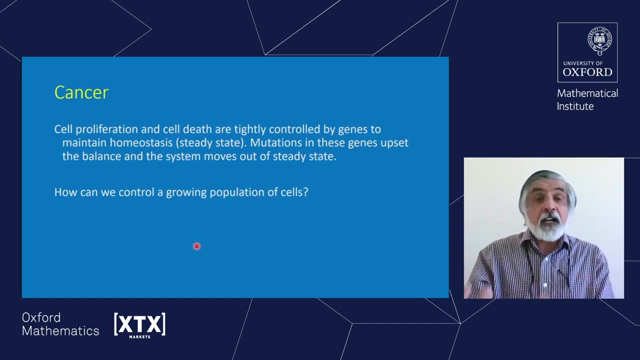 And cells proliferate, divide to compensate for that death, And you have a balance- the birth balances the death, and you have something called homeostasis or steady state. What happens in cancer is that a group of cells, through mutations, their properties change. 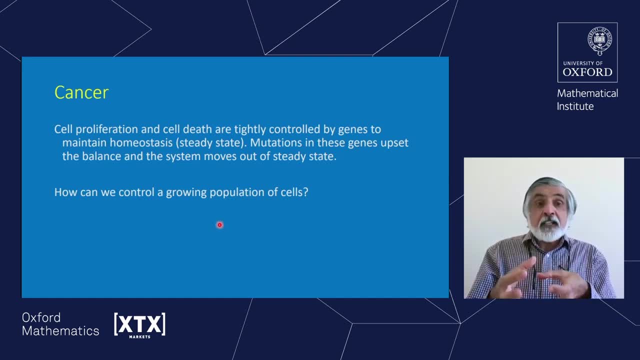 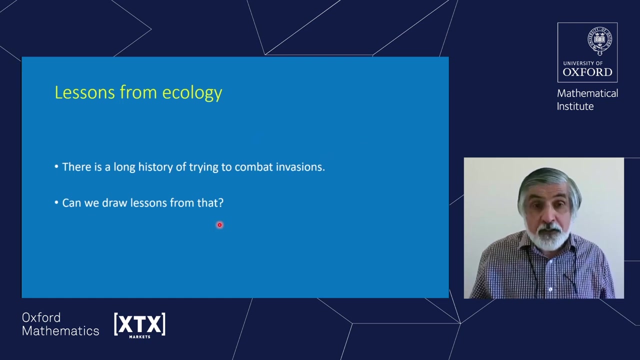 So that this balance of birth and death is upset And the net result of that is you get a growth. So the question in cancer is: how do we control this population of cells that are growing, that are actually invading our body? Well, in ecology there's a long history of analyzing invasion. 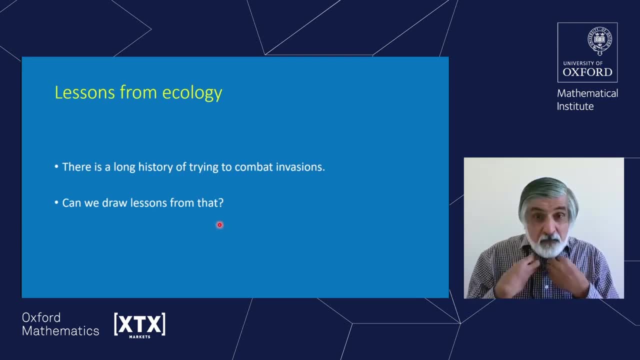 So if we think of cancer as an invasion of our body by cells, can we draw lessons from ecology? So one of the invasions that the UK experienced and is continuing to experience is the squirrel invasion. So this is the red squirrel, the indigenous squirrel, the host population. 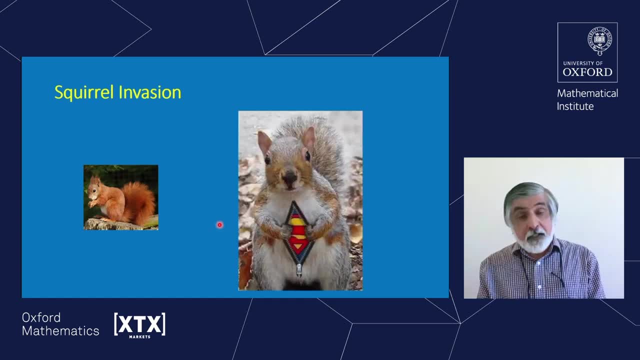 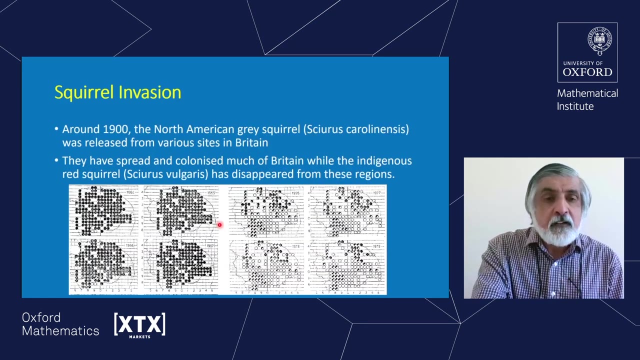 And in last century this character appeared. The grey squirrel imported from the US and the grey squirrel has invaded the red squirrel's territory. So I apologize for the very bad quality of this very old drawing drawing. so here we see, the southeast part of England. there's the coast there and in 1964 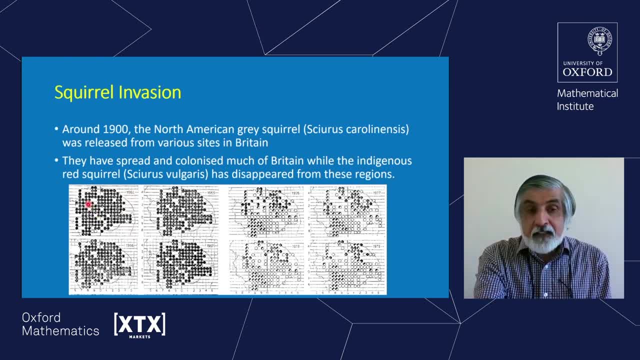 these black spots are where people have seen red squirrels during that year, and then this is 64,, 65,, 66, 67 and then 75, up to 79, and you can see, going from here to here, the red squirrels have begun to disappear and that's because they've been replaced by the grey squirrels. 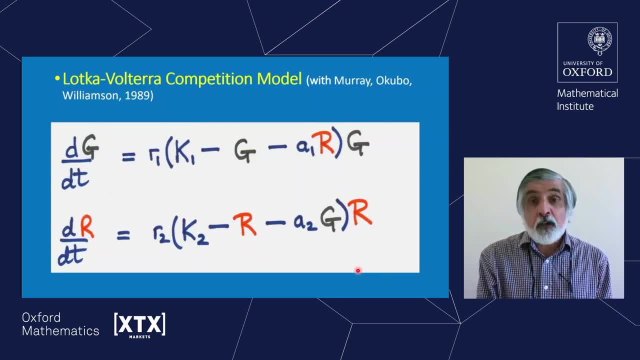 So this is something I worked on actually when I was a postdoc with Jim Murray, Akira Okubo and Mark Williamson, and we developed actually a Lotka Volterra Well known competition model to try and understand this invasion. So in these equations here, 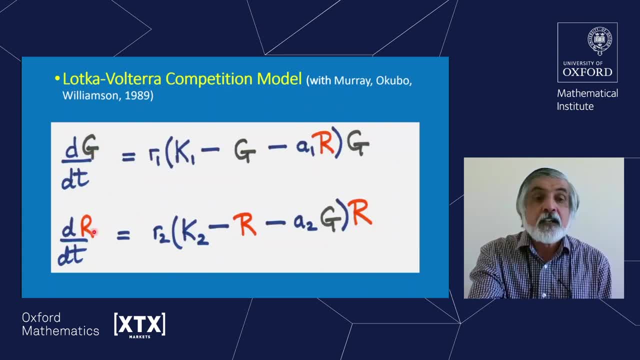 G is the population of grey squirrels, R is the population of red squirrels and T is time. So what do these equations mean? Well, let's look at the red squirrel, because that's the home team. Okay, so every other parameter, every other thing: R1, K1, R2, K2, A1 and A2- these are all positive. 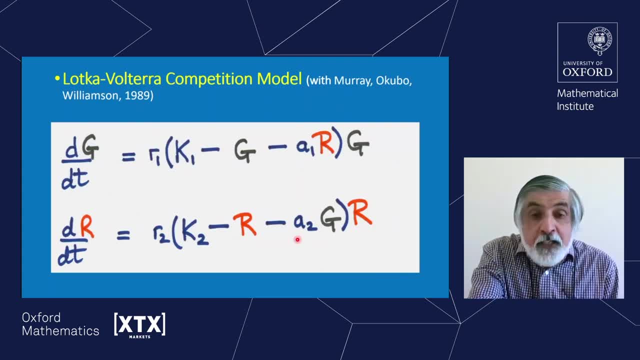 fixed values. Okay, so suppose we just had this term. so R2 times K2 gives you some number, positive number multiplied by R. So let's consider that first of all We'd have dr by dt is something positive times R, That means you have exponential growth And in fact exponential growth. 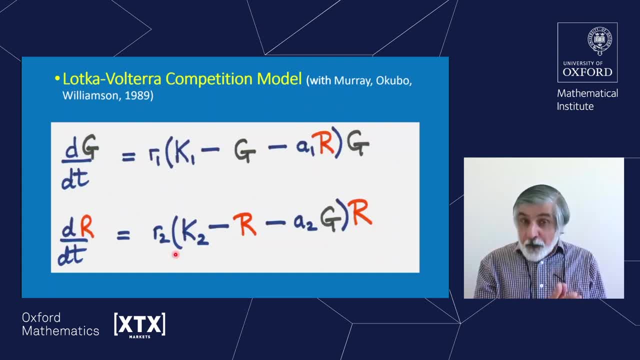 is a pretty good description of how a lot of populations start to grow. But of course, populations do not grow to infinity, because as they start to grow there's competition for resource and you'd expect the growth rate to decrease. The simplest way to model that is to use this equation. So let's look at the red squirrels: R1, K2, A1 and A2.. 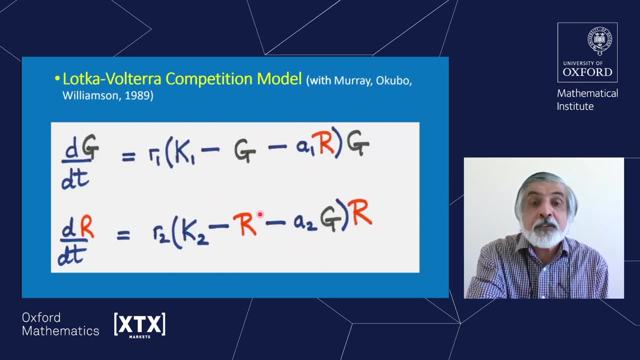 That is to put this term here in. So what this term is saying is that as the population increases, the growth rate, instead of being R2 times K2, becomes R2 times K2 minus R. It decreases because of the presence of the reds. Now, here we have a competition, and so the 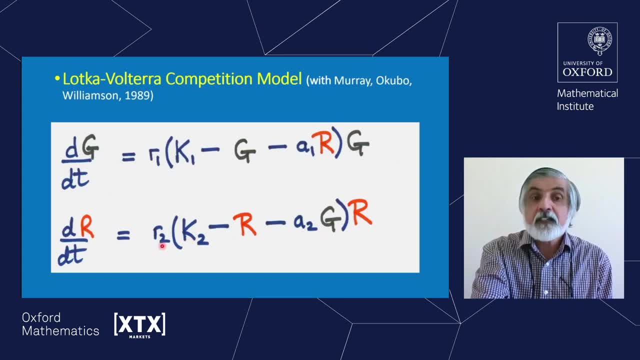 greys also decrease the growth rate, So you can think of this as competition for resources that decrease the growth rate, And the same thing for the greys, And if we think of the greys as being better competitors than the reds we'd have, this is bigger than this. 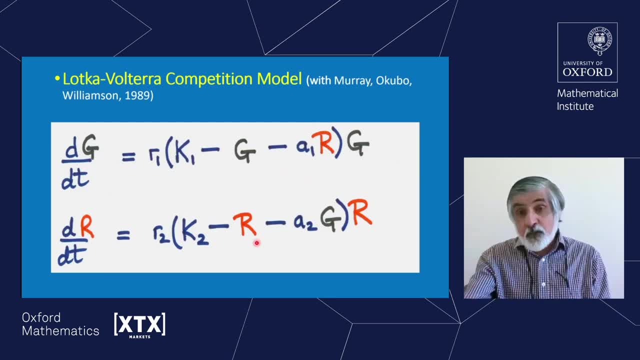 Okay, so then, on top of this, we would have diffusion, which haven't put in here, but we would have movement of the greys, movement of the reds, So let's see how this system with movement in it behaves. So this is a video that was in fact generated by a 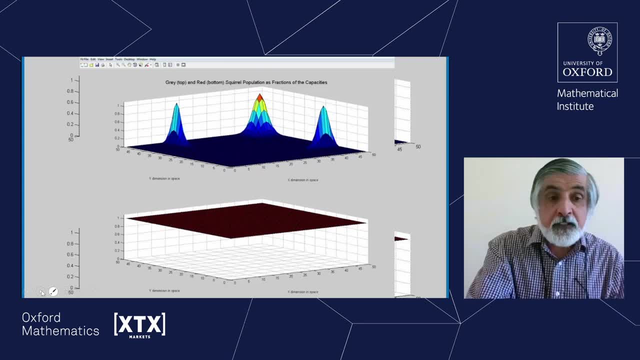 former graduate student of mine a long time ago, Anthony Connor. So what we've done here? we've scaled the populations to lie between zero and one. So here we have the red squirrels: they're all at population one. The grey squirrels are at population zero, except for some pockets. 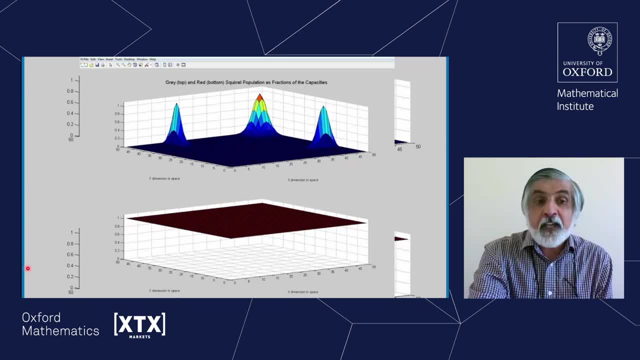 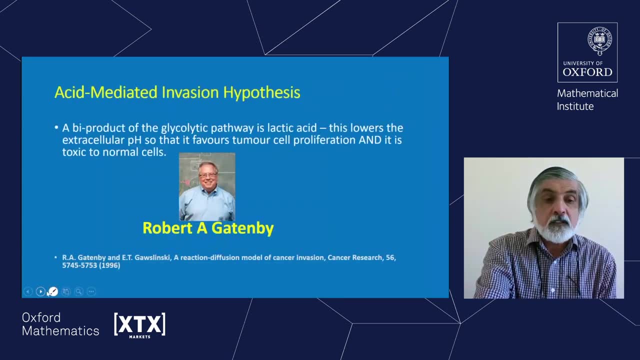 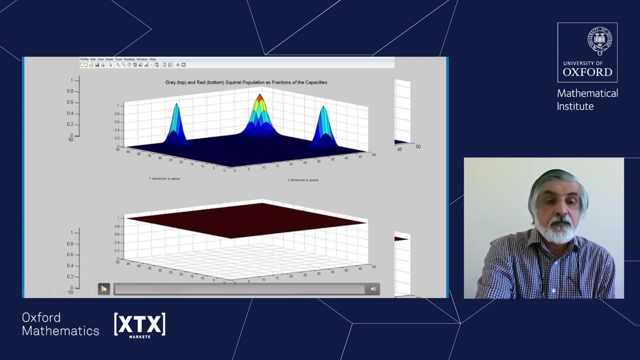 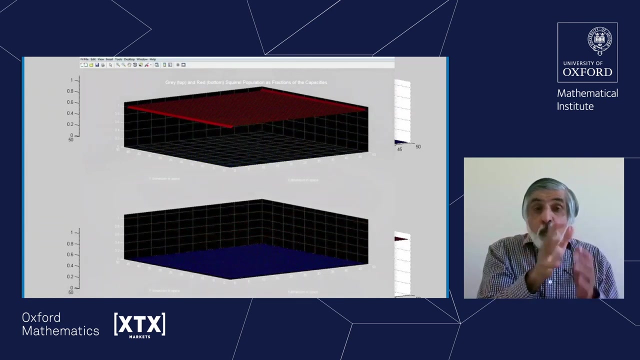 here at population one, And then we're going to ask what happens if we run this model. So we run the model and what you see happening is waves of the grey squirrels out-competing the reds. So in the end, the grey squirrels are now at one and the reds are at zero. 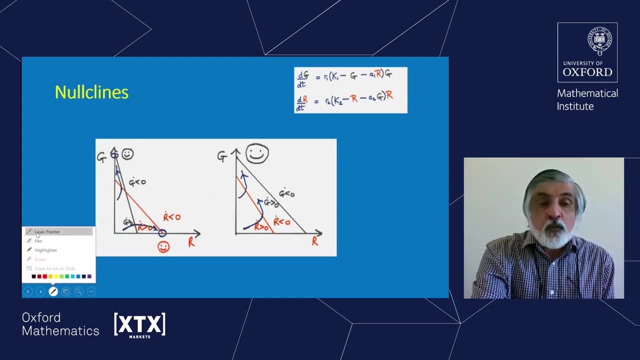 So let's try to understand how it was that the greys out-competed the reds, And the way to do this. you go back to these equations here and we look at something called the null clines, and the null clines are where these derivatives are zero. 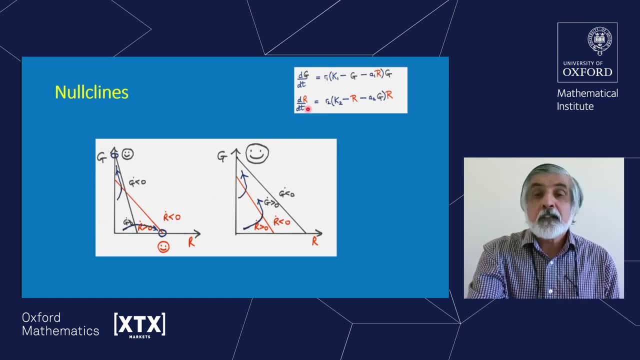 Okay. so if we look at the r equation, the r by dt is zero. if r is zero, which is this line here? or if this is zero, and that's this straight line here. Likewise, for g, we have: either g is zero or this line. Okay. so if we look at these two lines, 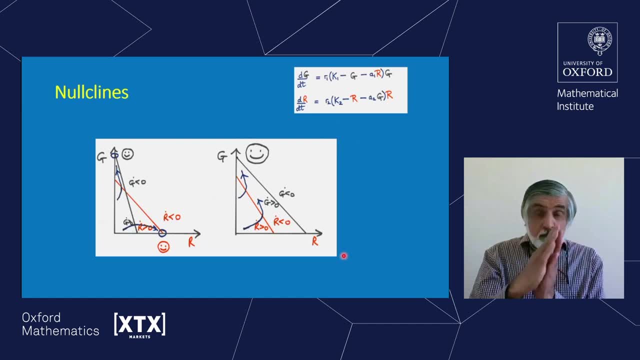 these are two straight lines and they can look differently depending on the values of k 1, a1,, k2, and a2.. They could look like this, or they could look like this, or they could have other combinations. Okay, so let us look at this one to begin with. 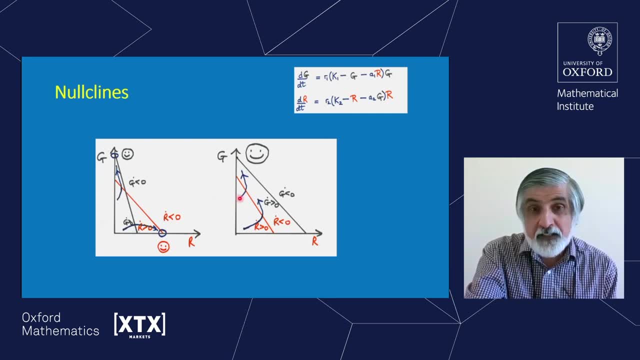 And suppose we're sitting here. so we've got some greys, a small number of reds. The greys have already come into the domain. Fix on the domain and see what's going to happen Now. our dot here is shorthand for derivative. 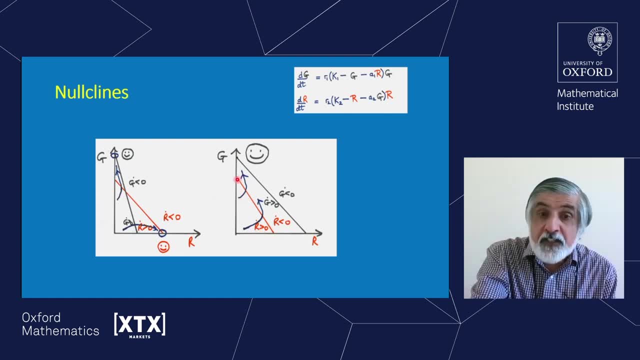 so at this point we are below this line where dr by dt is zero. So these are small, which means this is positive. So dr by dt is positive, so r will grow. Also, dg by dt is positive because we're below this line, so g will grow. 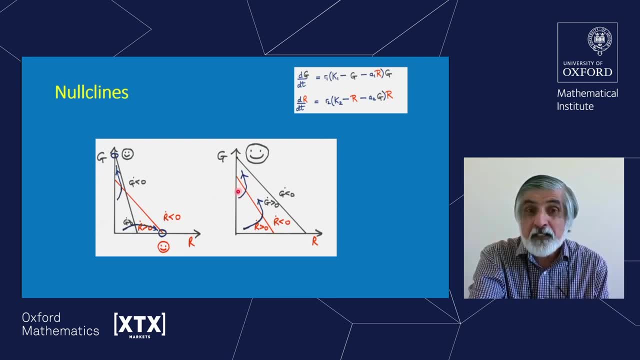 So the net result will be: if g is growing and r is growing, we'll move like this, Now, crucially, because the red line is below the grey line or the black line, here we cross the red line first. When we cross the red line now, the sign of dr by dt switches. 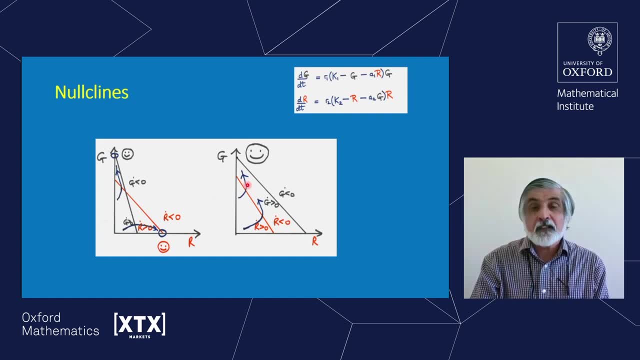 and the r by dt becomes negative, which means r starts to decrease. but we're still below the black line, so the grays are still increasing. So we go off like this and we reach this point here where the red squirrels are zero. this gray squirrel. this is supposed to be a very happy. 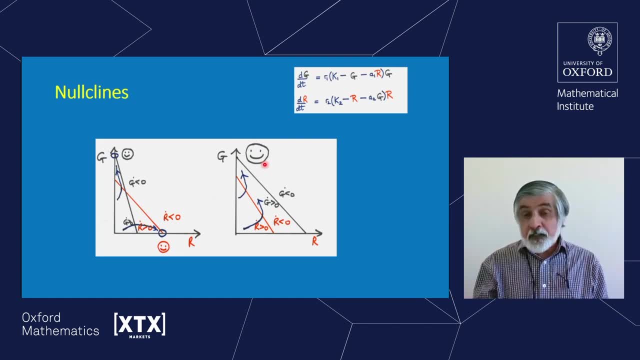 gray squirrel and we have had competitive exclusion. So suppose we now think: well, let's save the reds. and there've been lots of campaigns throughout the century- last century and this century- to save the red squirrel. Part of those campaigns are: let us cull the gray squirrel. 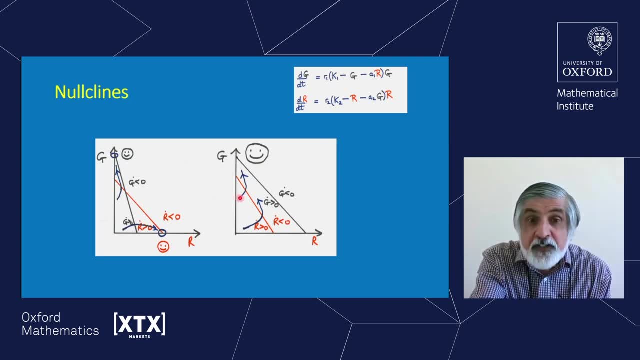 So we cull the gray squirrels, which means we decrease the population, but the red squirrels are still increasing. So we go off like this and we reach this point where we have the gray squirrels. So we've culled a lot of gray squirrels. what's going to happen? 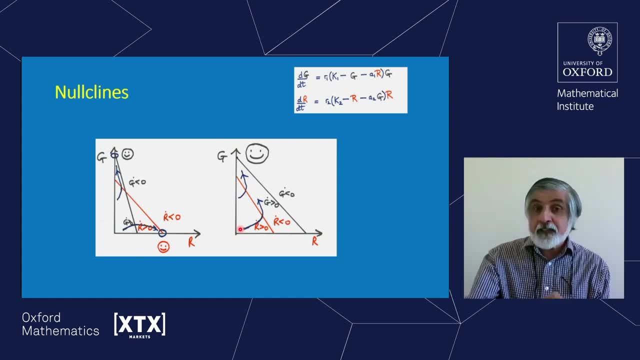 Well, we're below both lines, both nullclines. so the populations will start to grow and we cross the red nullcline first, and so we go up and we finish up with all grays. So it hasn't worked. On the other hand, suppose these nullclines 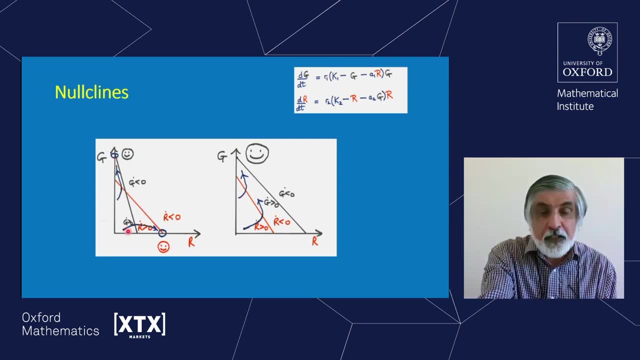 look like this. Now, here we are again. start off. here we're below both lines. both g and r increase. we cross the red line first, which means r starts to decrease, and we go to here: happy gray squirrels, red squirrels, are all dead. 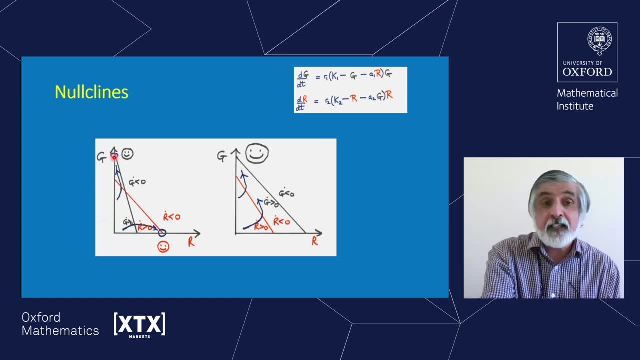 Now let's do the same experiment we did on the right hand side: let's cull some grey squares. We move down to here. Once again, we're below both null clients. so both G and R will start to increase. but now there's a difference. We 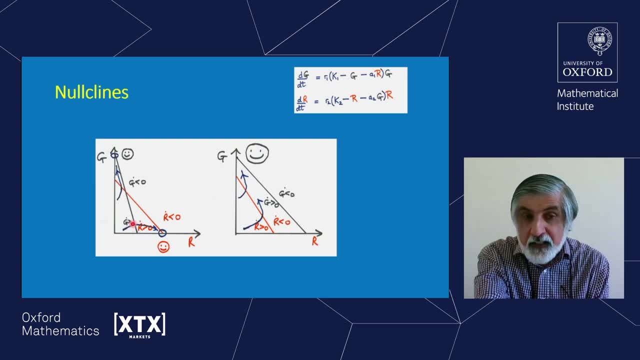 cross the black line first, which means that the greys start to decrease, Then we move down to here and we finish up excluding the greys and happy red square. So two points to note from here. the same experiment gives different results Here. 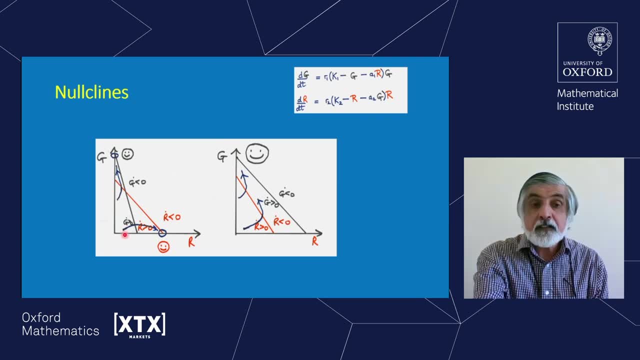 grey is 1.. Here red is 1.. Second thing to notice is that if we are in this situation here and then we think that there's a difference in the number of Culling, will never work. We have to do something else. We have to change the 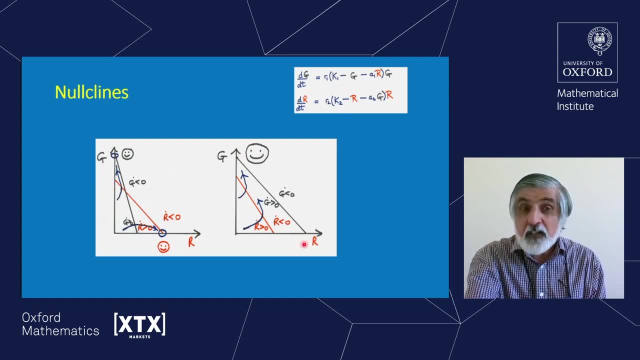 slope slopes of these lines so that they intersect like this. Now, the slopes of these lines and their intersections are determined by these values here. So what we would have to do is we have to somehow make the red squirrels better competitors than the grey squirrels, Or make the environment such that the red 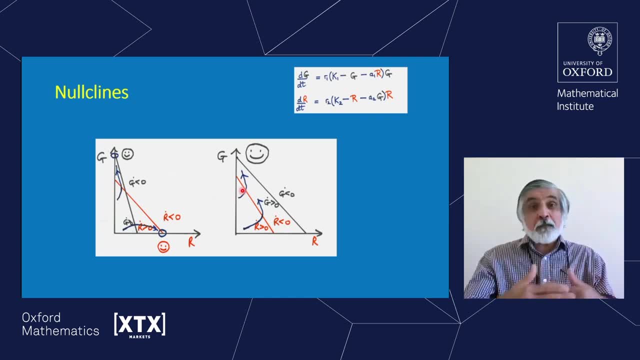 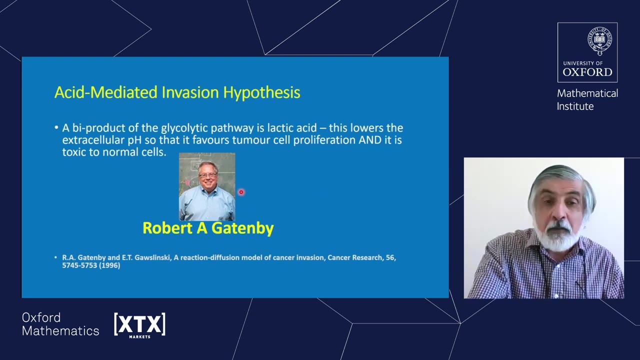 squirrels are better suited to the environment than the grey squirrels, So that's the insight we get out of this. These insights have been used by my friend and collaborator, Bob Gatenby, who began life as a physicist and now is a cancer biologist and actually a radiologist. who's 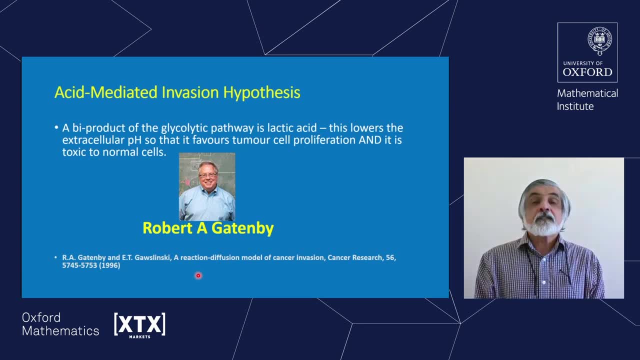 at the Moffat Cancer Center in Tampa. So it's well known that cancer cells sometimes use a metabolism that is less efficient than normal cells use, And this metabolism is called anaerobic metabolism and this is called the Warburg effect. Now, basically, if we have lots of oxygen, if our cells have lots of oxygen, 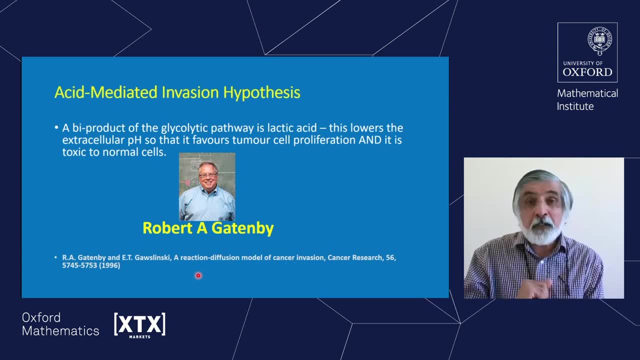 we use aerobic metabolism and that produces lots of energy. If oxygen decreases, the cells then use anaerobic metabolism and that involves glycolysis And that is lower production of energy gives lower production of energy. And what Warburg noted was that in some 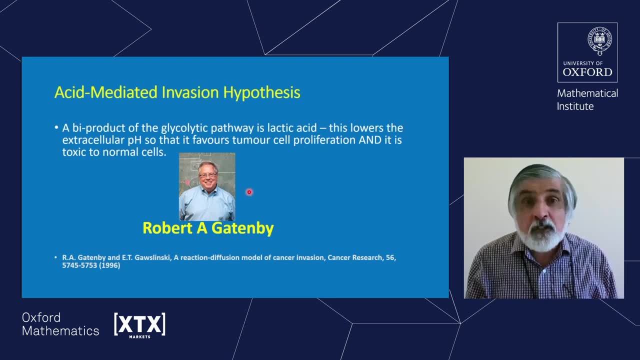 situations where there is enough oxygen, tumour cells use this anaerobic metabolism. So that doesn't seem to make sense. Why would you use a lower energy generating system in a competition? So Bob's theory was the following, or his hypothesis was the following: 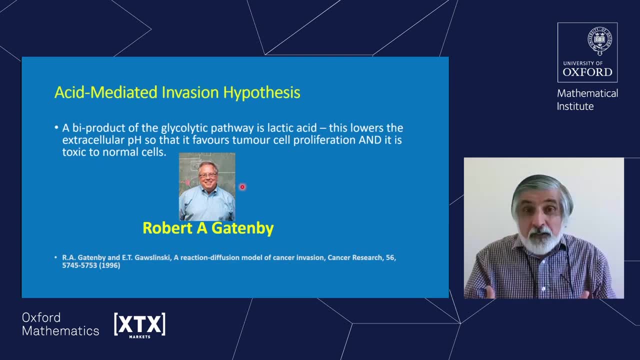 He said that okay, you've got these invaders By using the glycolytic pathway. one of the byproducts of the glycolytic pathway in the metabolism is lactic acid And that makes the environment acidic And the acidic environment favours tumour cell division and it's more toxic to not be oxidised. 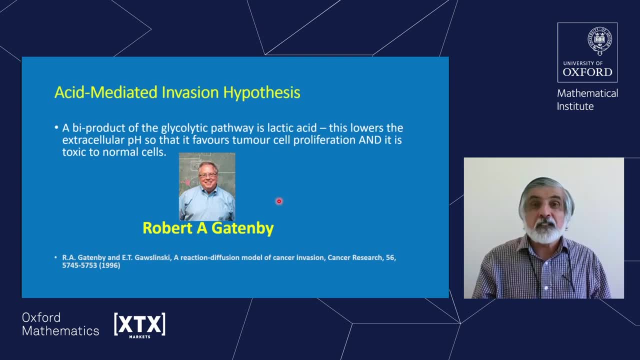 normal cells than to the tumour cells. So what the cancer cell is doing is it's changing the parameter values to make the environment more suitable for it than for the normal cells and to help it to invade. So he wrote down a system of equations. 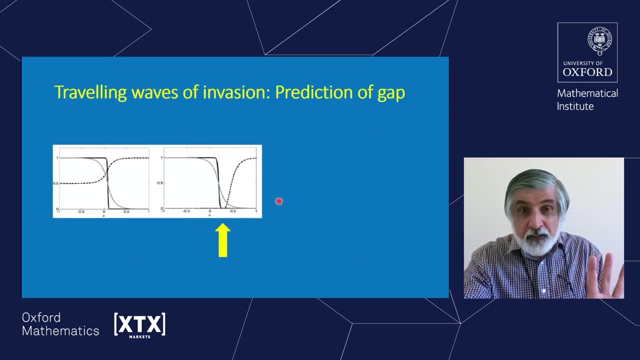 a bit different to the ones we've just looked at, but the essence is the same: a competition model- and he solved this competition model, and so what we see here is this is in space, and this is his model, where this black line are the tumour cells that are invading. 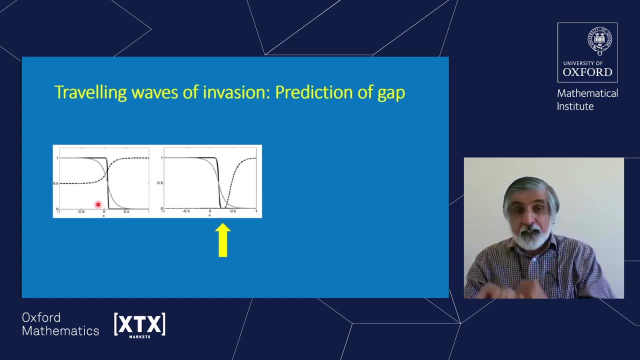 so they're forming a travelling wave that's moving along like this. this is the acid that they're producing and these are the normal cells. so the normal cells initially were at one everywhere and they're still at one here, because there's no tumour cells but the tumour. 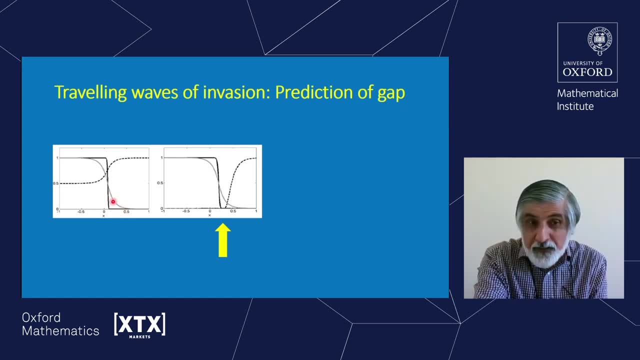 cells have started to invade, They're producing the acid. the acid is changing the environment, making it more suitable for the tumour cells and for the normal cells, and so this will grow. You see what's happened here: the normal cells they were at one, now they've come down to 0.5.. 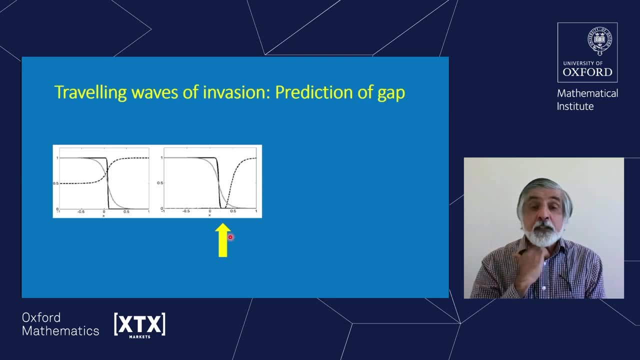 In other parameter regimes, it was even more dramatic what he found Here. you see, it started off again with normal cells everywhere, and then he introduced some tumour cells, and then he introduced some tumour cells, and now these tumour cells are invading and they have pushed the normal cells to extinction. 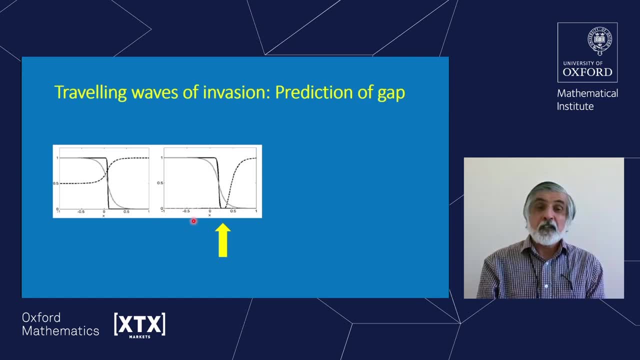 so this is competitive exclusion. Now, what he found, which was a novel thing, was this strange business here. Here there are no cells. So the prediction of this model was that if tumours are using acid to mediate their invasion, there should be a gap with no cells. 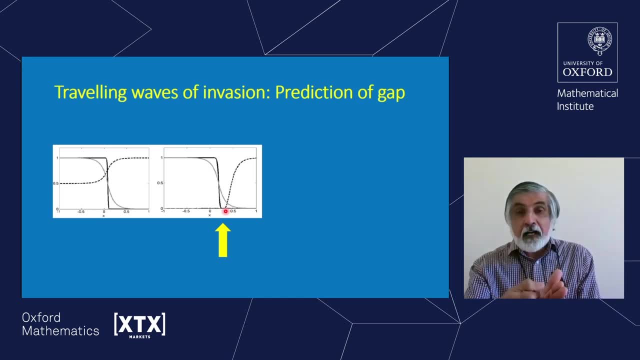 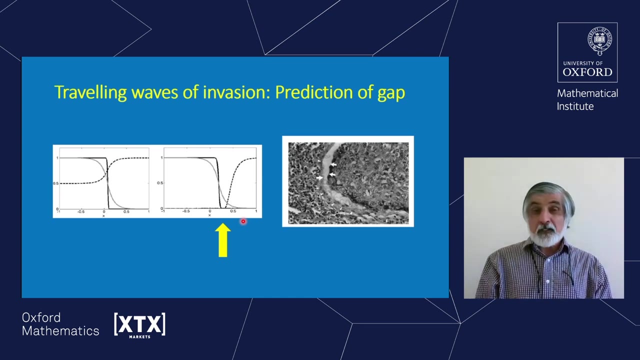 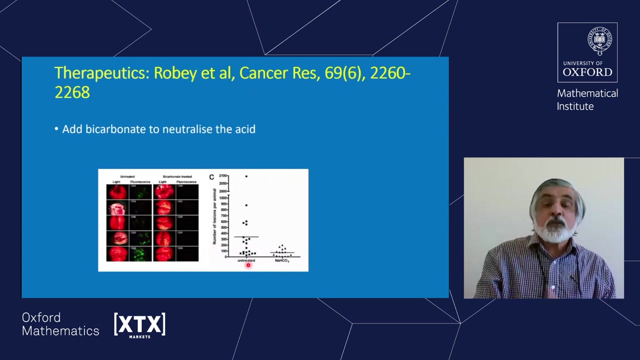 between the invading front of tumour cells and the regressing front of the normal cells. So then Bob went and looked at some human head and neck cancer, And in several of these head and neck cancers he found a gap. So this leads to a very obvious next experiment. 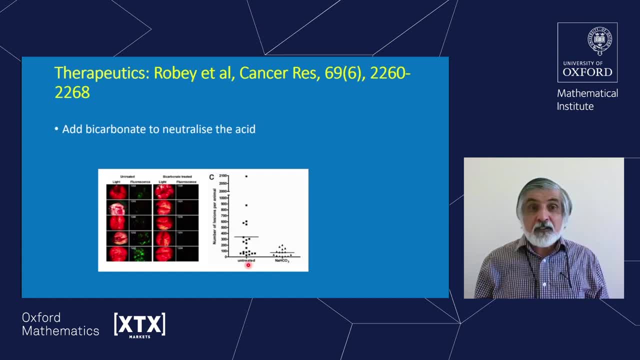 If the tumour is changing the environment and making it acidic so that it can invade, then what would happen if we neutralised the acid? And this is an experiment by Enrobe and various people. This is done on mice, So mice were injected with tumours. 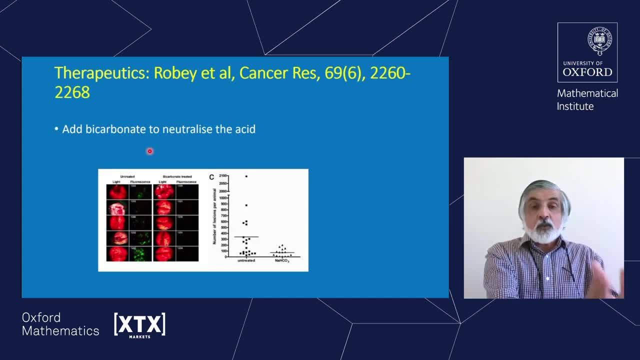 The control mice were just left to do their own thing. The treated mice were given water that had bicarbonate in it, And then what they looked at was how many metastases were formed. In other words, from this initial tumour, how many groups of tumours broke off and invaded. 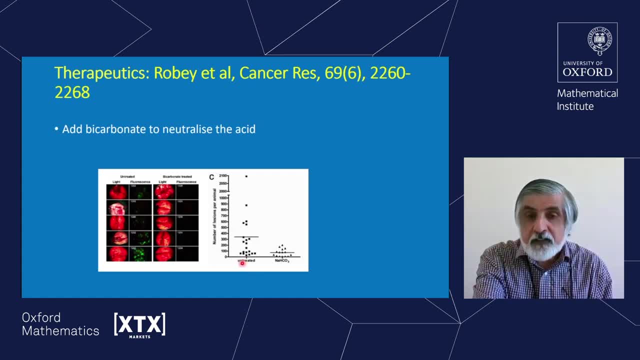 And what we see here: in the untreated, here's the average, and in the treated, here's the average. So the treatment didn't stop, totally stop the invasion, but it significantly reduced the invasion. So the mathematical model which tested and validated the hypothesis led to these experiments. 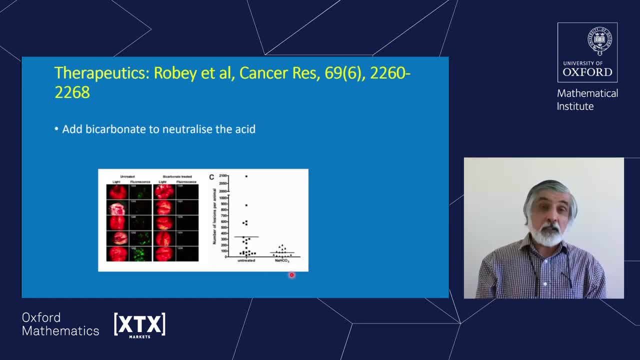 that again validate the model. Now this is in mice and mouse is a model. We're humans, we're not mice. And then the question is: just because it works in the mouse, can it work in the human? We've got a completely different metabolism. 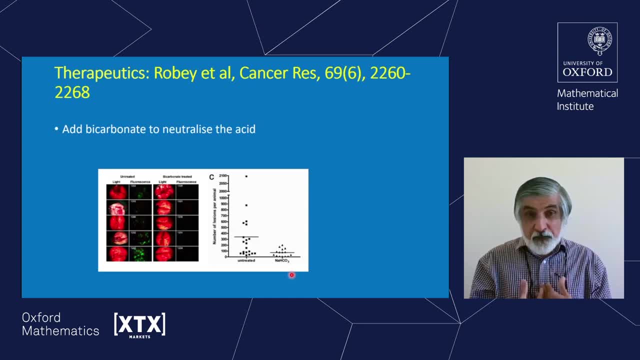 completely different immune system. lots of things are different between us and the mouse, But this work has actually instigated a whole series of experimental work and modelling that this group at the Moffitt Cancer Centre are doing, and they continue to work on the role of metabolism. 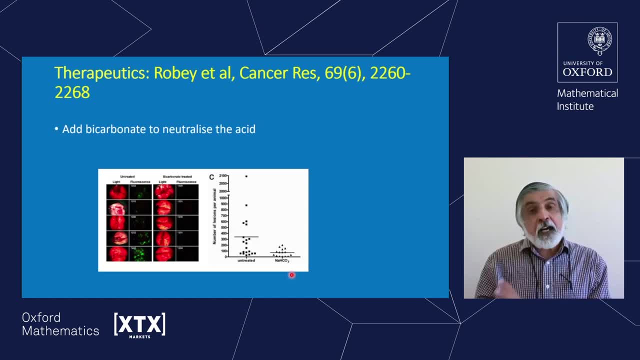 in cancer progression and can we alter metabolism in order to stop cancer invasion? And they work at the cancer at the Moffitt Cancer Centre and in fact there are a group of seven or eight full-time mathematicians working with clinicians and the experimentalists, headed by Sandy Anderson. 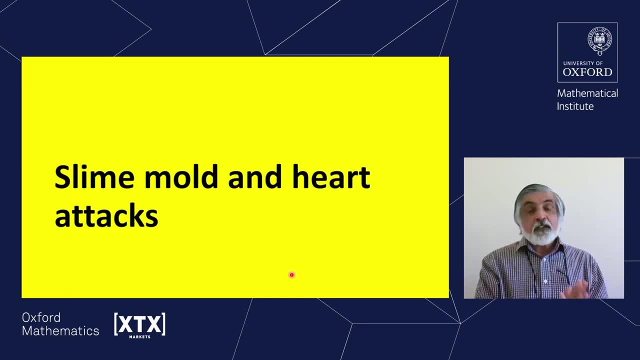 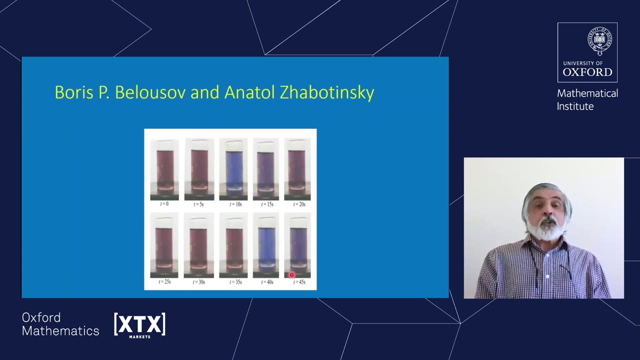 So I'm now going to move on to something to do with slime mould, which is developmental biology, and heart attacks, which is physiology. So, but before we do that, we'll do a little bit of chemistry. In the 1950s, Belousov. 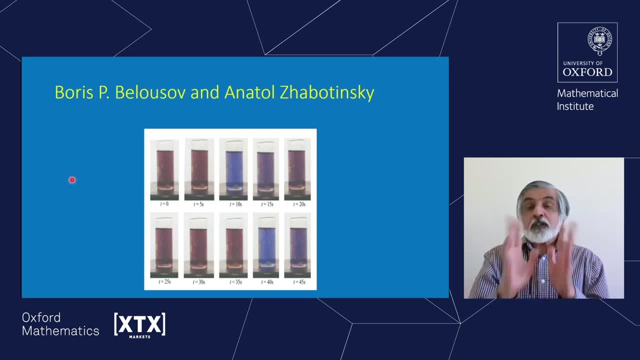 and then later Zabotinsky worked on this chemical problem and this was a chemical reaction where the chemical here, this is time, and it is red, pink, and then it goes blue, and then it goes back to red, and then it goes blue, and this keeps on happening. 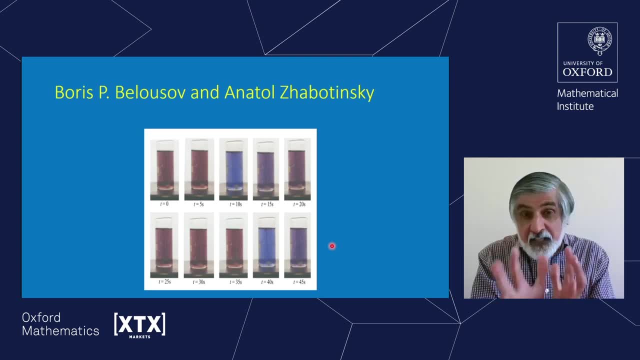 What's going on here? This chemical that they're looking at, this chemical reaction is a redox reaction, where the chemical, when it is oxidised, it's in a certain colour and when it is reduced, so deoxygenised, it's a different colour. 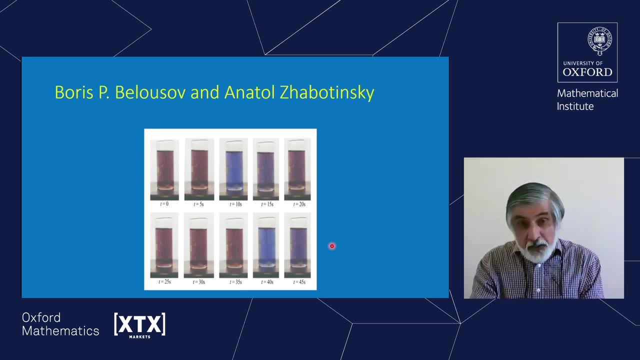 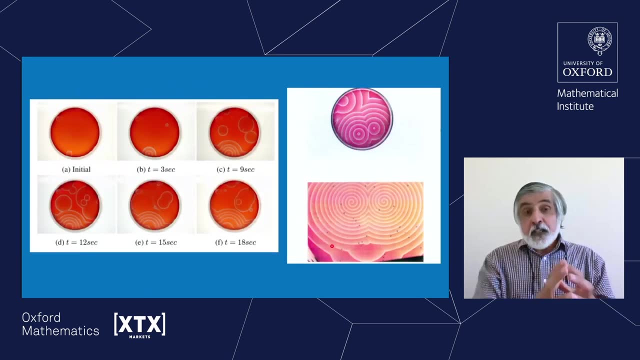 So what we're seeing here is oxidation reduction, oxidation reduction, etc. etc. So how is this happening? And in fact, if you look at this in a dish, you get all you get waves, like you did for the squirrels, but these are much more interesting. 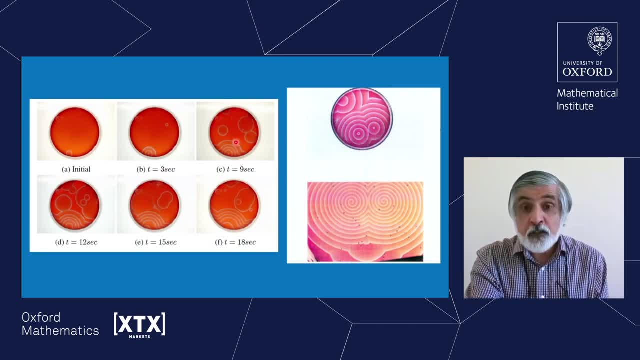 You get these what are called target patterns, because they look like targets. You can get here's target patterns and here are spiral patterns. So what's happening here? These patterns propagate and they break up and they form spirals. So go to the internet. 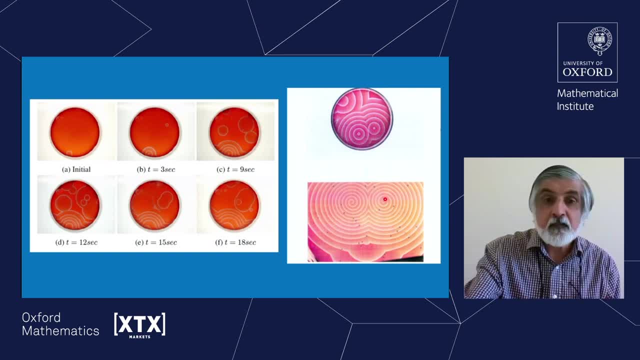 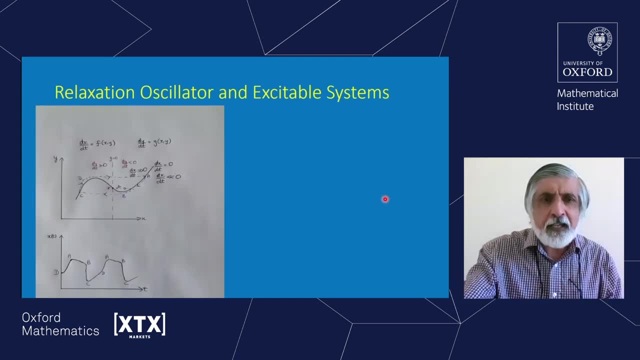 and you can see videos of these. Okay, so how can we understand that? So lots of people have developed models for these and this is the sort of the field noise model and a very, very simplified version of it. So we now think in this set up. 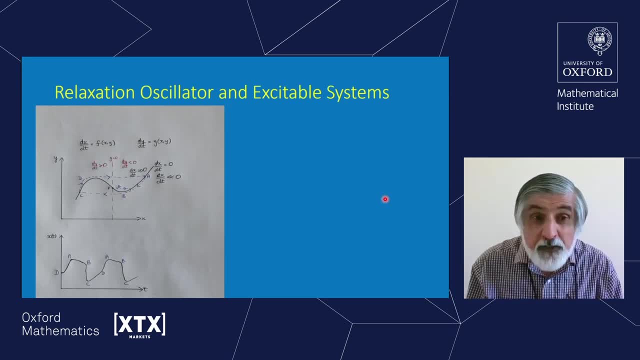 X and Y are two of the chemical players and we draw the nullclines And the nullclines for X. well, here's one nullcline- it's a cubic- and the nullcline for Y. I've just drawn it very simply here as a straight line. 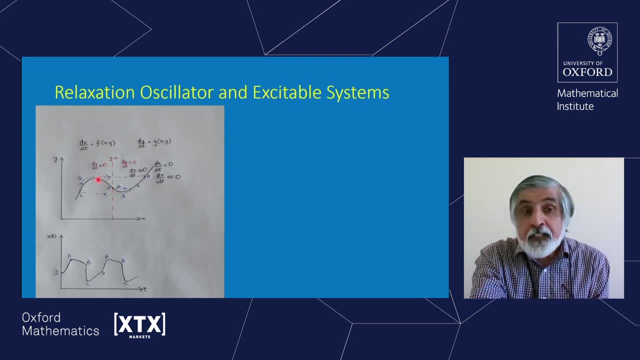 The important thing is that the nullcline only intersects along this branch, So this nullcline could be like this: doesn't really matter, The key thing is it intersects along here. Okay, And it turns out in this system when you are above the black nullcline. 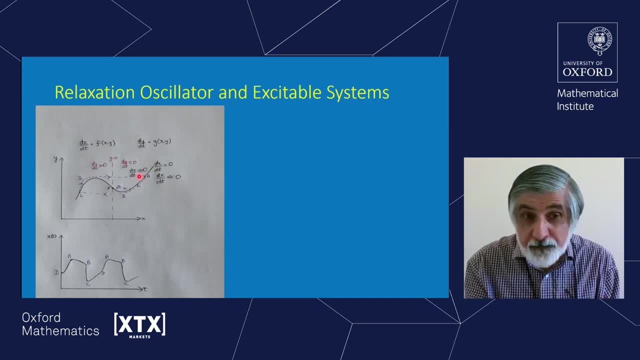 not only is dx by dt positive, it's very positive. Remember, the nullcline is where the derivative is here. So one part of the nullcline, the derivative, will be positive. on the other part, it will be negative. One of the differences between this and the previous model. 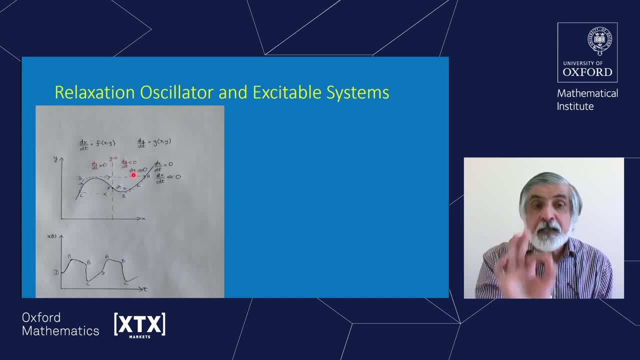 is that this X derivative is very big on this side positive, very big on this side negative. So suppose we start at this point P. So at this point P dy by dt is zero, dx by dt is zero. this is a steady state, So the system would stay there. 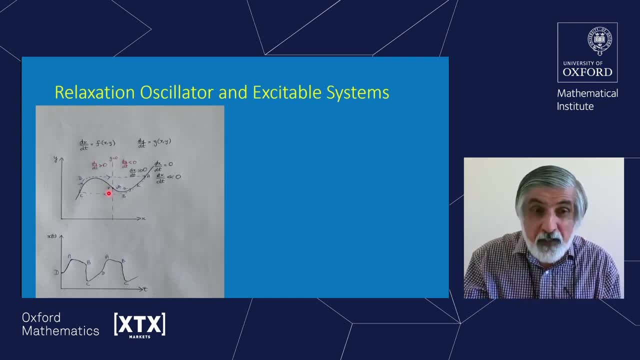 nothing's changing. But in a biological system there will be small fluctuations, So suppose there's a small fluctuation that pushes us to Q. So if we look at Q, dy by dt is negative, so Y will decrease. dx by dt is positive, so X will increase. 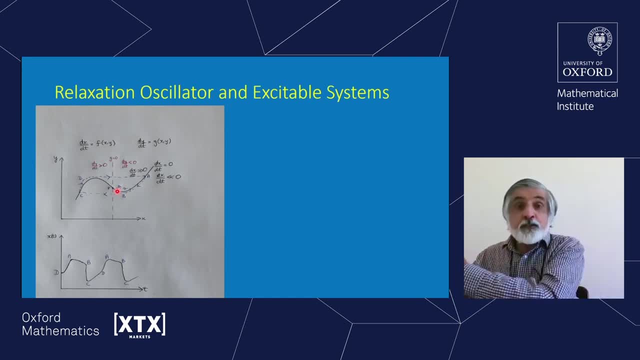 but it's very big, so it will increase rapidly. So the net result will be: we shoot to here and we cross the nullcline, and now dx by dt is negative. So we start to go down And the thing is that we stick to the nullcline. 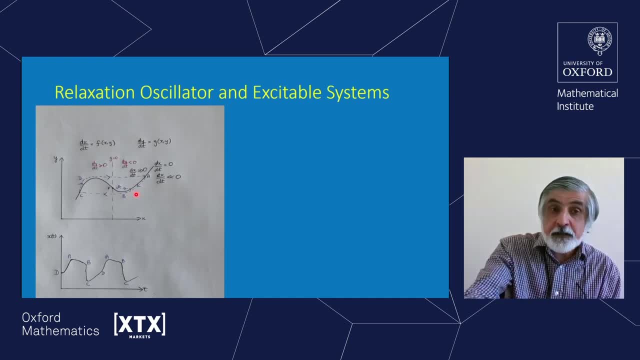 because if we try to fall off the nullcline, dx by dt is very large negative. it'll push us back. So we go down and then we reach the point B. So ideally we would like to stick with the nullcline. so we'd like to move up. 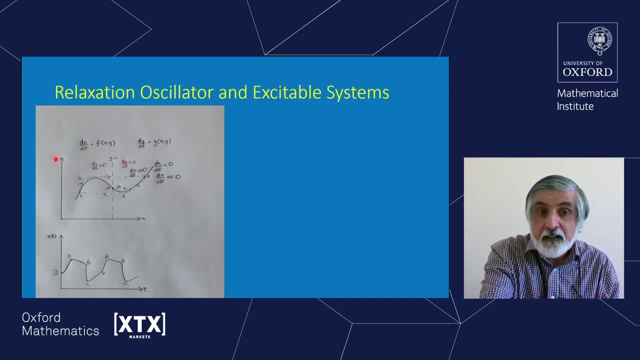 but that would mean Y increasing. But look, Y doesn't increase, Y decreases. So we fall off the nullcline and we shoot across to this point. And now, at this point, dy by dt is now positive, So we increase. Go up to here. 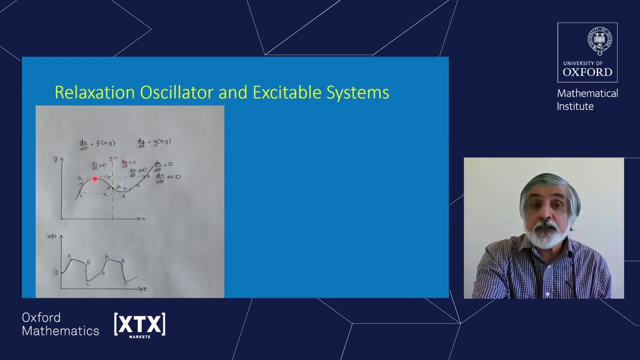 reach this point and then, at this point, we fall off the nullcline again, shoot across to A and keep on and on going. So what does X look like as a function of T? Let's look down here, Say, at D: X increases very quickly to A. 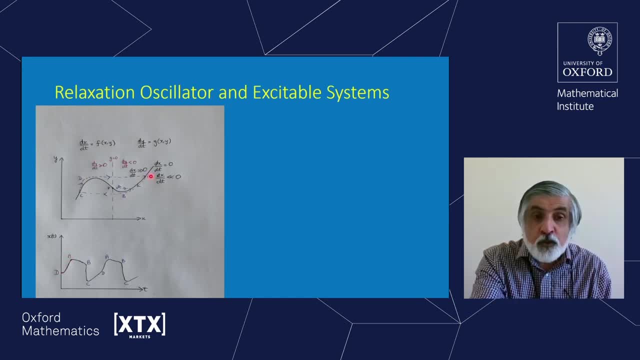 so it shoots off to A, slowly decreases to B, slowly goes down to B, quickly decreases down to C and slowly moves up to D and keeps on going And that's the oscillation. So there'll be other chemicals that will be oscillating out of phase with this. 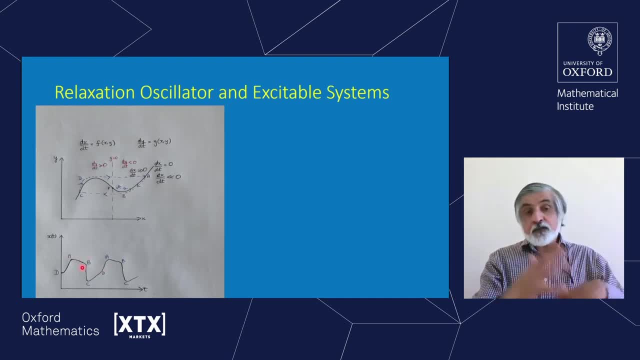 So when this one is high and you've got, say, an oxidized version and the reduced version is low, so you have one color and then they swap. then the reduced one is high, the oxidized one is low, you have a different color, And this keeps on happening. 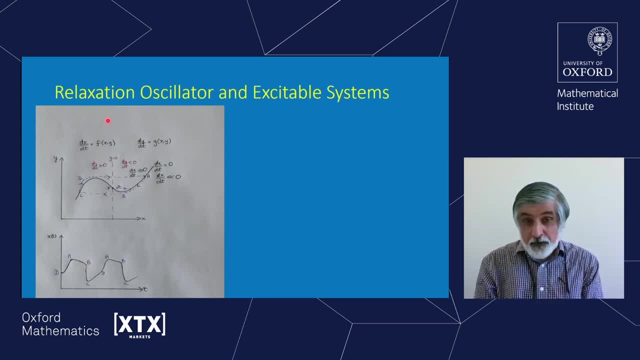 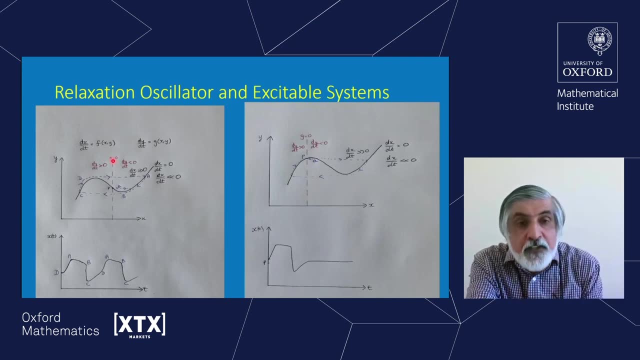 And this is called a relaxation, relaxation oscillating, Okay. Okay, Now what would happen instead of this nocline intersecting here, Suppose it intersected here on this branch, but near this maximum. Now, suppose we do the perturbation again from P and we move to Q. 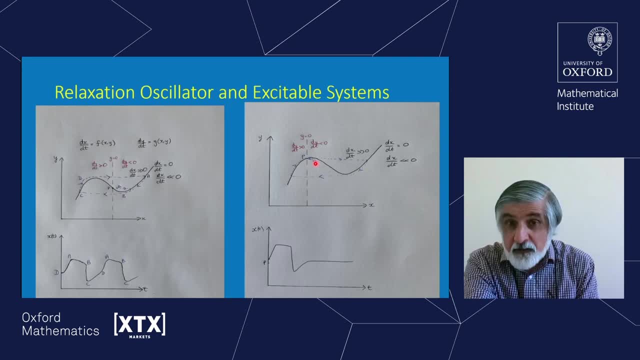 So at Q dx by dt is negative because we're below the x nocline. So x will decrease, y is negative, y will decrease and we'll shoot back. But suppose instead we move to here in our perturbation. Now dx by dt is positive. 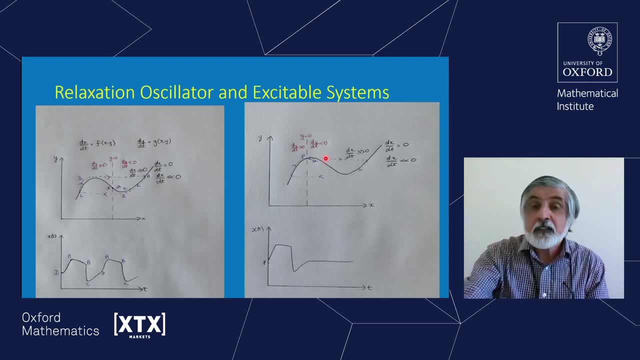 and we shoot in the opposite direction: Move right across to here, come down to here, move right across to here, again up to here, and then we stop at this steady state. So, crucially, here we have what's called a threshold phenomenon: If we make a small perturbation. 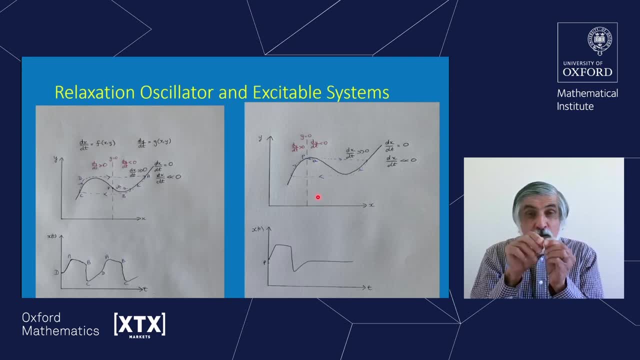 we go back to where we started, but if we breach a threshold, we then have a big excursion before we go back, And that is this type of behavior, This type of behavior here That's called an excitable system. Now, one of the amazing examples: 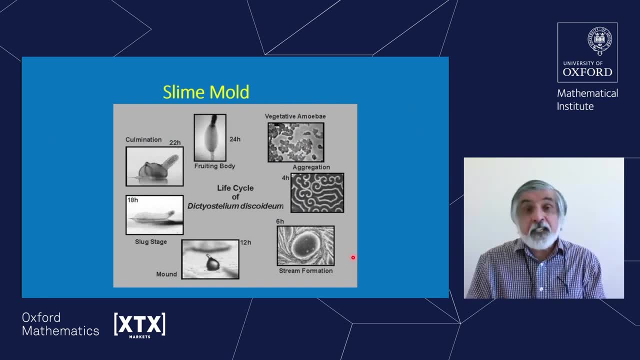 where we see an excitable system is in something called the slime mold, and again, I would urge you to go and look at movies of this on the internet. So slime mold are single celled creatures who live around you, enjoy life, eating, reproducing, but then times become bad. 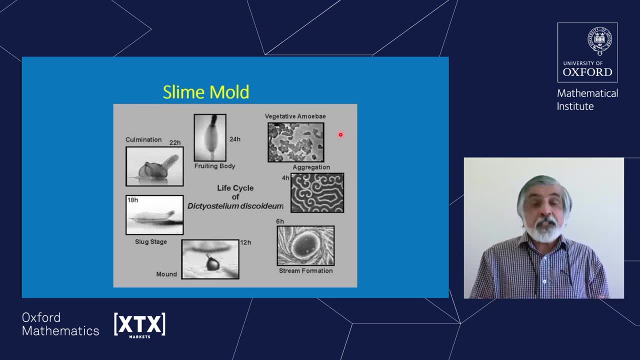 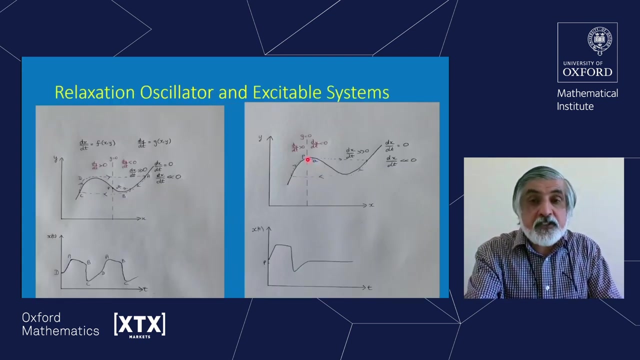 and they run out of food. So what do they do? Well, some of them start to secrete a chemical called cyclic AMP. This chemical diffuses and the chemical and cell combination is an excitable system, So that when this chemical comes to the next cell, 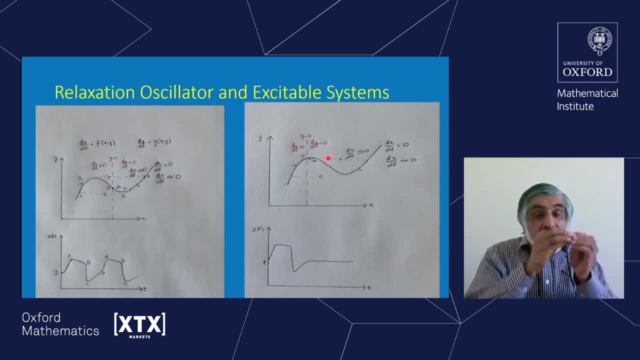 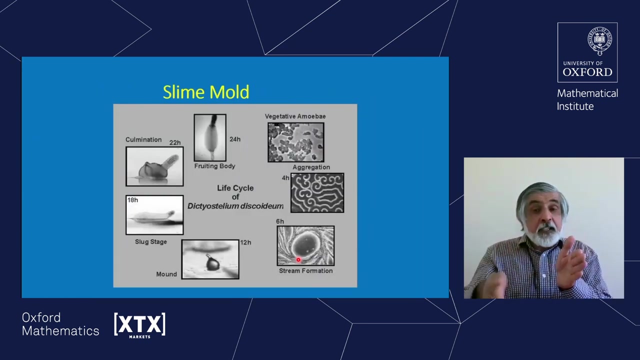 it perturbs it and so it then releases the chemical. and this is in time. but in space, as we saw here going back here, we get traveling waves, So this would be a traveling pulse. So in this way the signal gets relayed and these 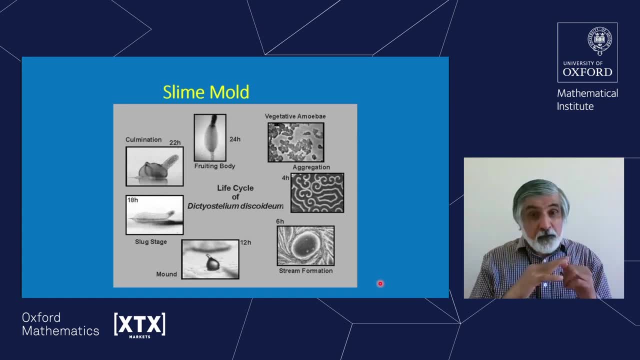 cells move up the chemical gradient and form these streams which eventually aggregate and form a slug, a mound and then a slug. So basically, this idea: you send out the chemical. and the reason to send out the chemical is to signal to all your friends: we've got to get together. 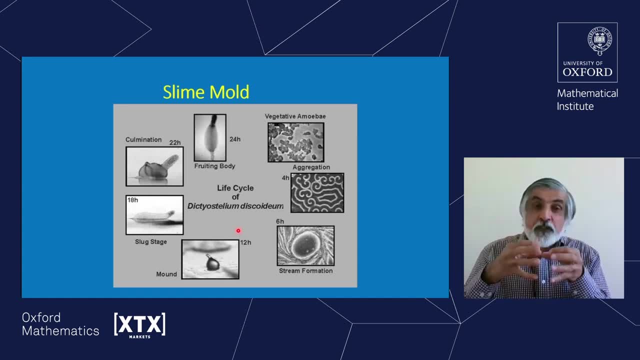 and form a slug. The importance of this slug formation is that when the cells come close to each other, they can exchange certain key proteins. that allows some of them to become stalk cells and some become spores. So what you get here is a fruiting body. 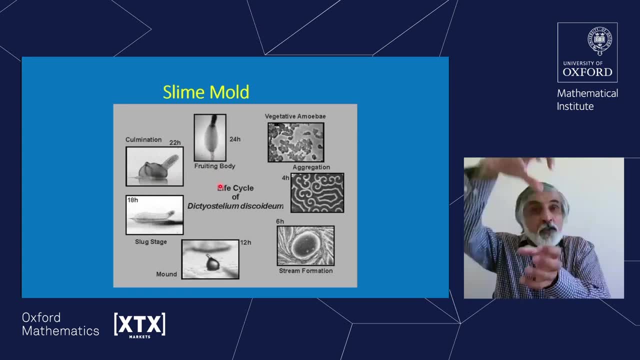 where these things grow up, and then you have spores at the top and stalk at the bottom, and the spore cells are the ones that survive. So an animal comes, pushes them away, or the wind comes, blows the stalk cells or the spore cells away. 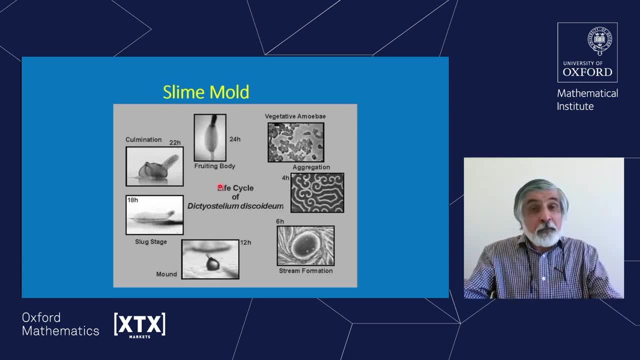 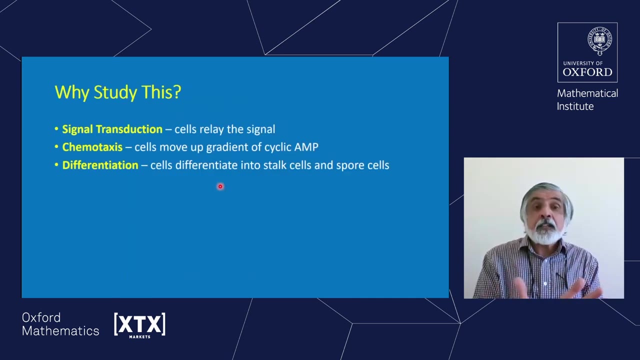 and then hopefully blows them away to a better environment where these cells can grow again. Now in the 1980s and 90s this was studied a lot because it had processes that are vital in higher organisms: Signal transduction, which is how you relay the signal. 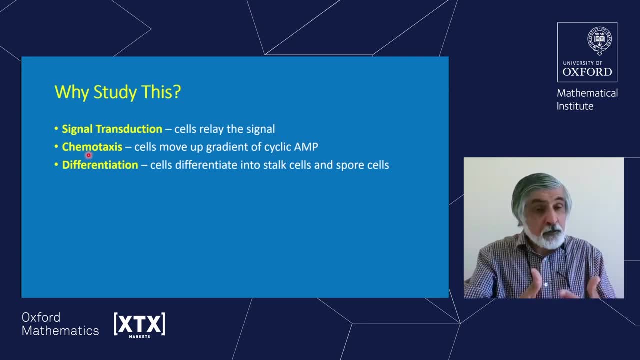 Chemotaxis, the movement of a chemical gradient which is very important in higher blood vessels, form in higher immune system, response to disease and differentiation of how these cells change from one cell type to another. These are all key processes in higher organisms, but the slime mold. 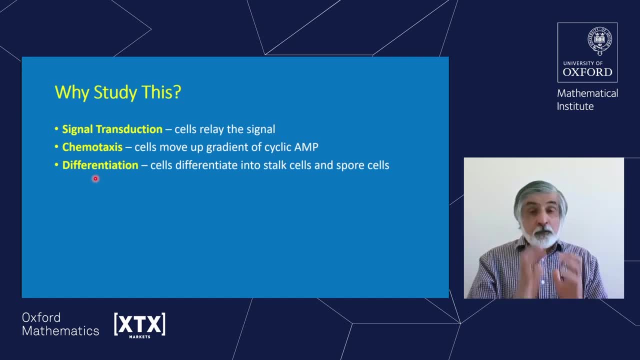 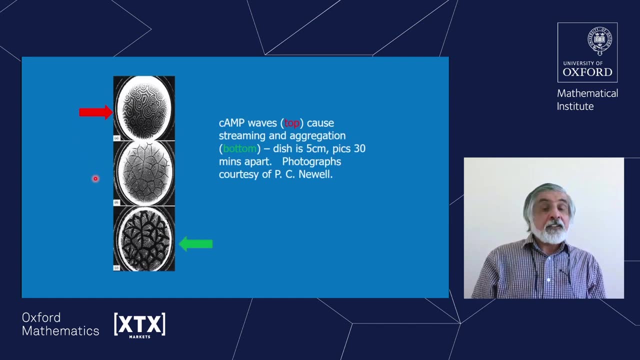 was a really good study, a really good model system to study this. And in fact, if you look at this in 2D, here are cyclic AMP waves and you can see they form spirals and target patterns, very much like the the Lussov-Zapotinsky reaction. 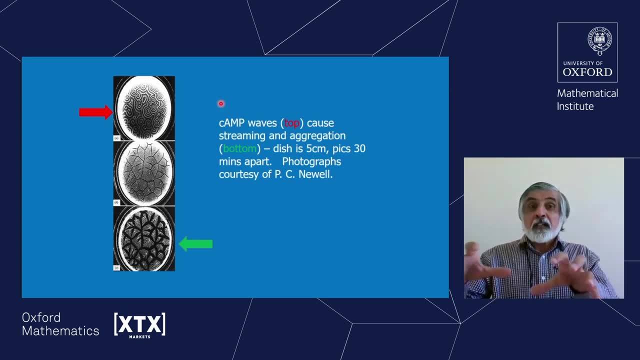 So you can see, here we've got a biological system, there we had a chemical system. they both exhibit similar patterns and from a mathematical point of view we see that there are several equivalences between them. And then here are the cells responding and forming the streams. 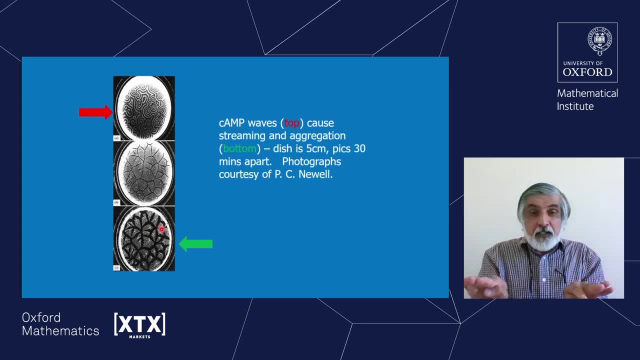 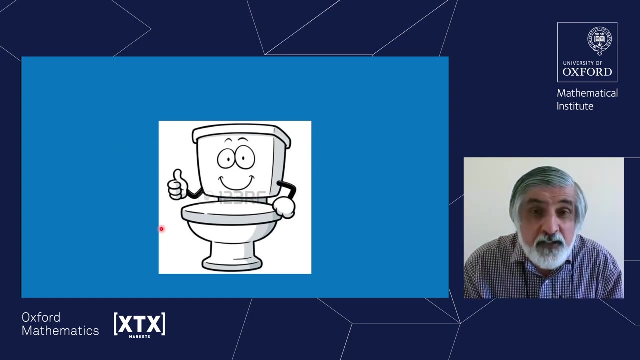 So we see the equivalence there between a chemical system and a biological system. So excitable systems are very important. Here's another example of an excitable system: a flushing toilet, The one with a handle, not the one that you wave at. Think about a flushing toilet. 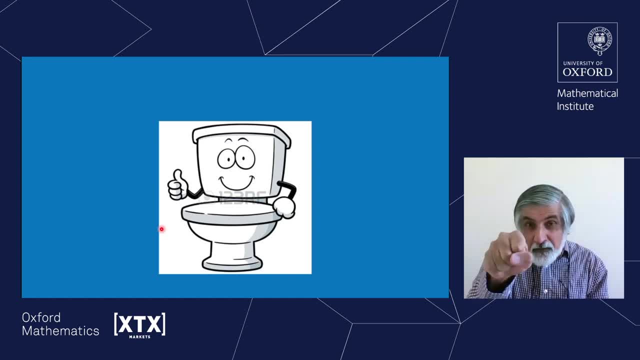 If you go along and you push the handle just a little bit, what happens? A little bit of water dribbles out, you perturb a little bit from the steady state and you go back, Pull the handle a little bit more and when you reach the threshold, 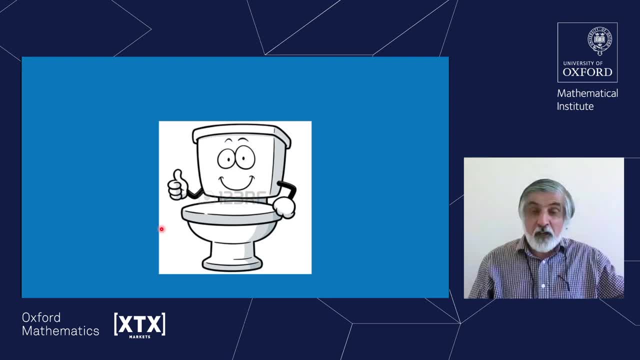 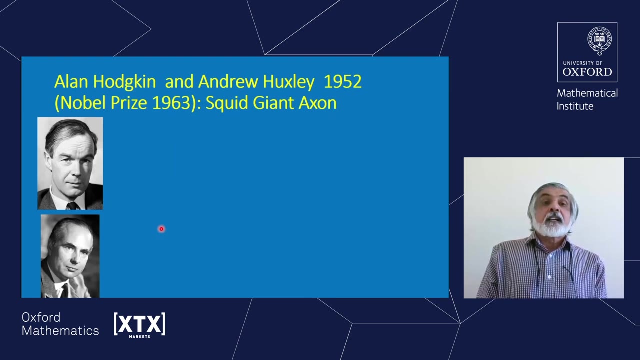 then, whoosh, a whole pile of water comes down and then you relax back to the steady state. So that is an excitable system. So moving on quickly. in 1952 Hodgkin and Huxley wrote a series of papers for which they won. 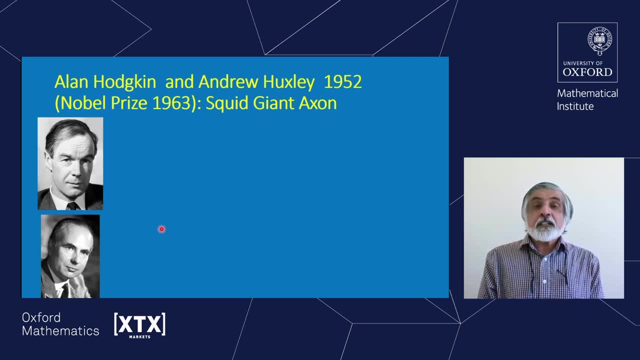 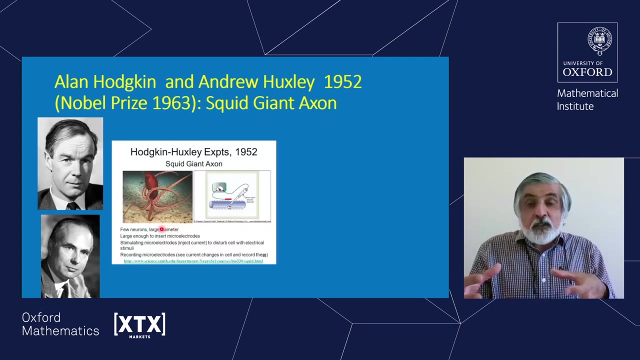 the Nobel Prize. some years later, They were looking at the giant, the squid giant axon. sorry, I nearly said it wrong: their giant squid axon. that's quite scary. this is the squid giant axon. So what does that mean? Well, basically axon. 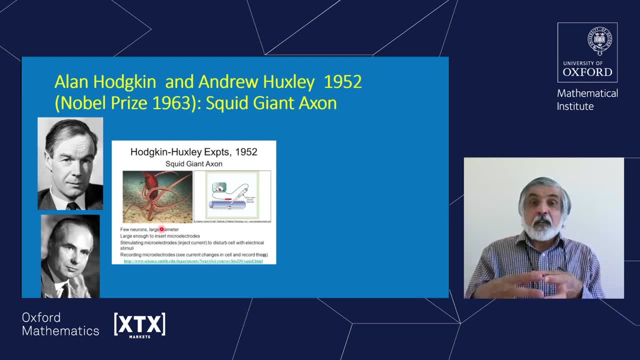 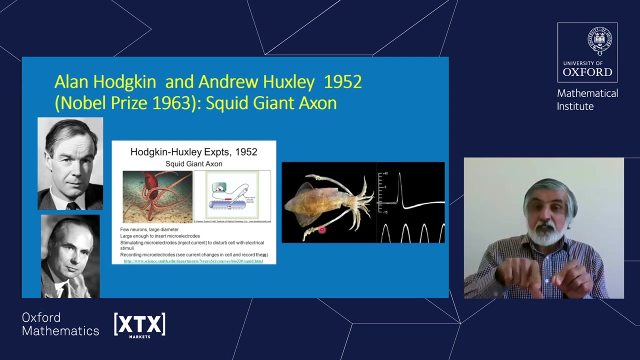 these are looking at the nerve cells, and the nerve cells communicate with each other via long protrusions that are called axons And the communication is electrical communication And basically what happens is you have an electrical pulse that bleeps in your cell and then that propagates. 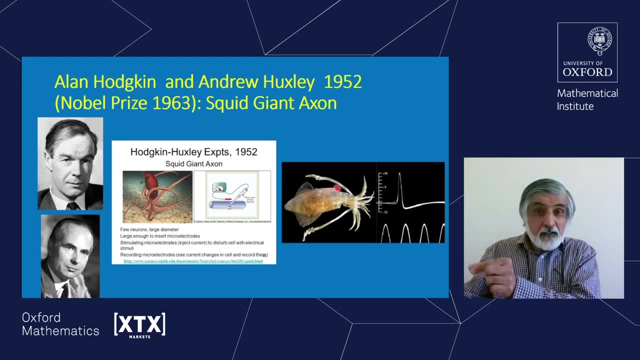 it kickstarts the next cell that pulses and kickstarts the next cell that pulses And in that way you propagate the signal And this work. their paper for this, their mathematical model for this, was a very complicated model of four equations and it was later reduced. 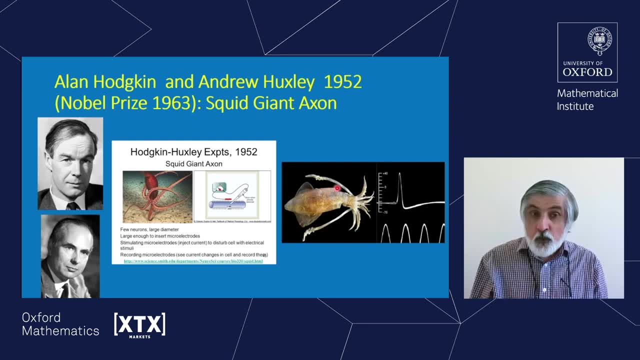 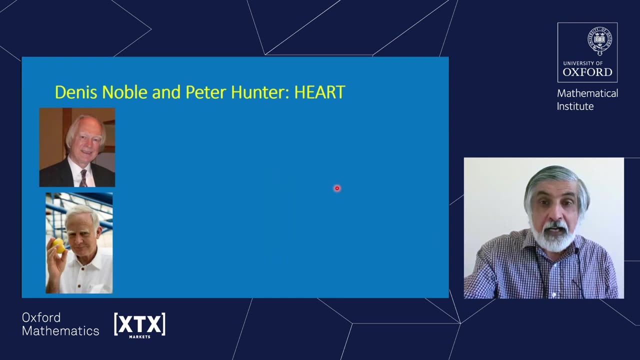 to two equations by Futsu Nogumo, who showed that this behaviour was identical to the behaviour we've just discussed in terms of the relaxation oscillator and the excitable system, And, in fact, there's been a lot of work on modelling of the heart. 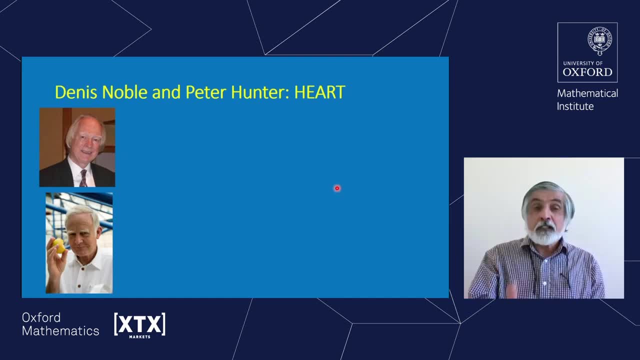 and in particular, people like Denis Noble and Peter Hunter, have done a huge amount of work on developing models of the heart because these excitable, so in the heart you basically have an electrical pulse that sweeps down the heart, that triggers a mechanical response that causes the heart to beat. 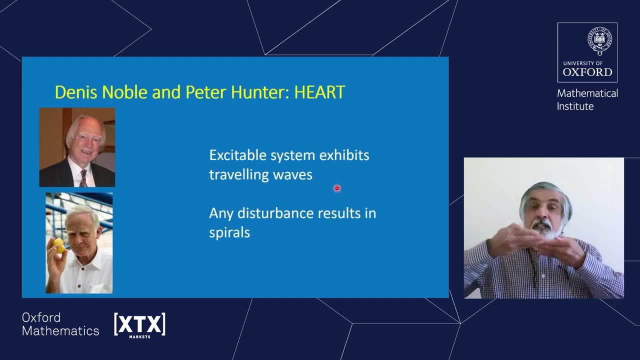 Now, as we've seen, these excitable systems propagate this signal. But if there is a bit of the heart that maybe has died, maybe there wasn't enough, there's a blood clot, so there's not enough nutrient getting to that bit- then, as this wave comes to that point, 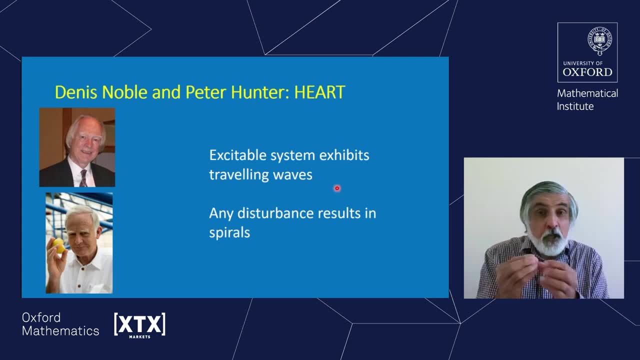 that point is going to have different properties to the rest. Therefore, the flow of this wave through that part of the heart is going to be a different speed and the wave will break up And, as we saw with the slime mould and with the um Bluzas-Rabatynski, 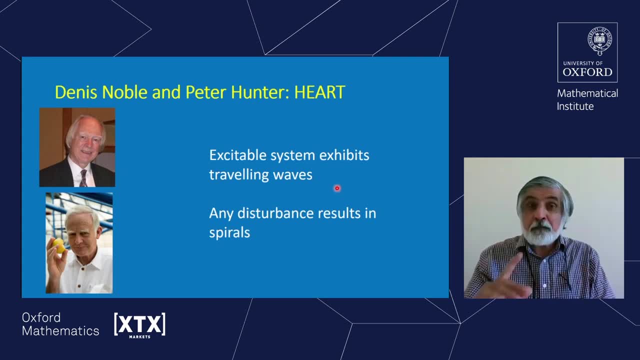 reaction. once these things break up, they form spiral waves And we can see that in the heart, and that means your heart would then try to beat, not as a coherent beat, mechanical signal, coherently beating the heart, but the signal would be a spiral signal, causing the heart to contort. 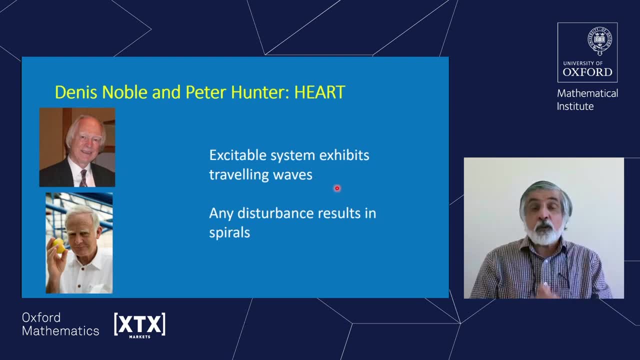 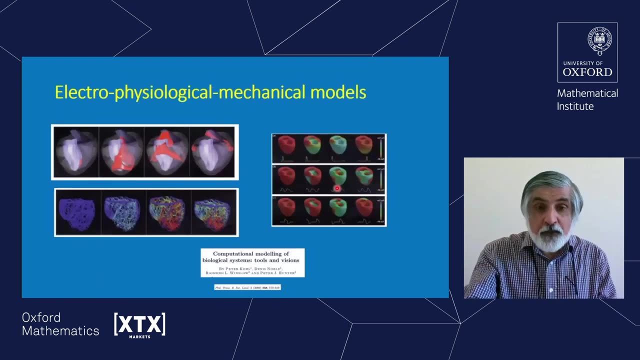 And so that can't be properly. that's called fibrillation And in fact these researchers and many other researchers have actually developed very, very sophisticated models of whole heart, models where they take into account a lot of them, the detail, anatomical detail of the heart. 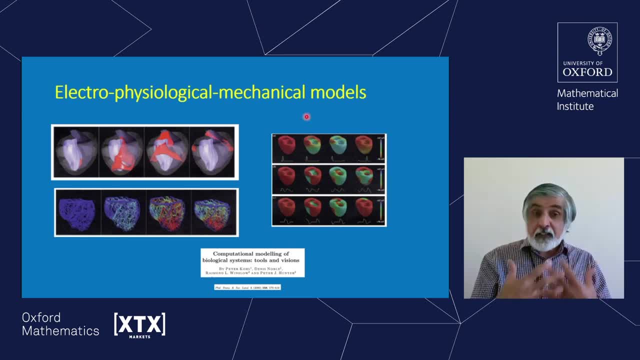 and the electrophysiology and mechanical aspects of the heart to see how you get these beats and how it is then that you can get fibrillation, etc. So and then you can use these if you're going to give a drug, some drug, and you want to make sure. 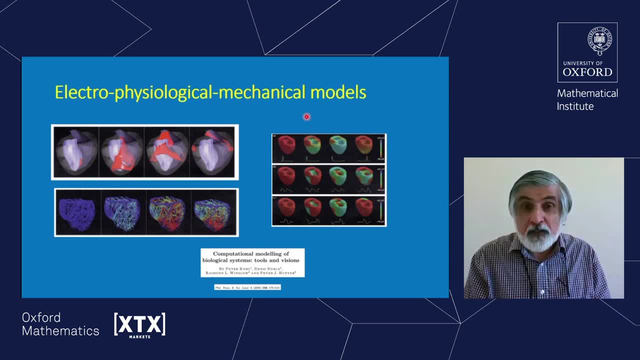 that that drug doesn't lead to heart problems. then you can see. well, if that drug affects the ion channels and therefore the electrical system and the excitable system, can we make sure that it doesn't lead to these instabilities that lead to defibrillation, that lead to fibrillation? 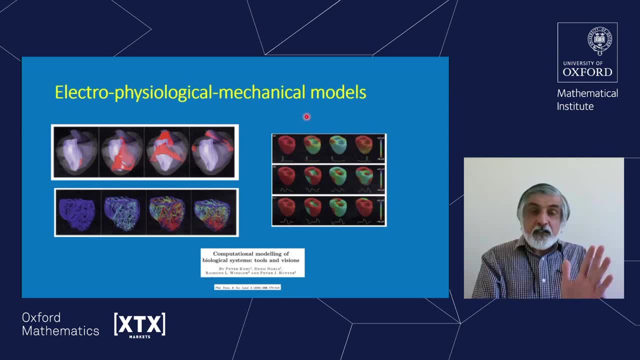 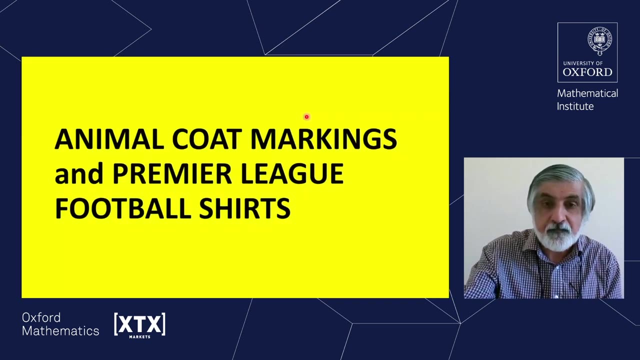 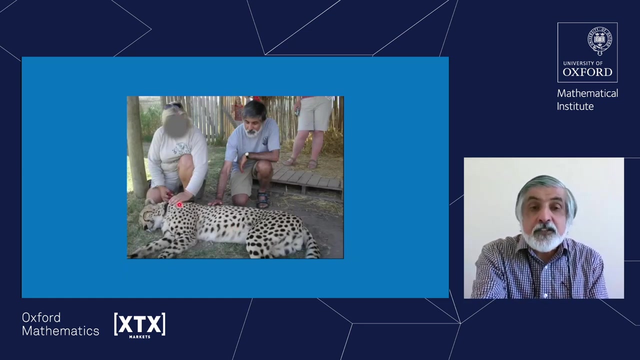 So what we've seen here, then, is phenomenon phenomena, a phenomenon that occurs in chemistry, developmental biology, physiology and plumbing. The last thing I'm going to look at is animal coat markets and football shirts. Okay, so here's an animal. It is a. 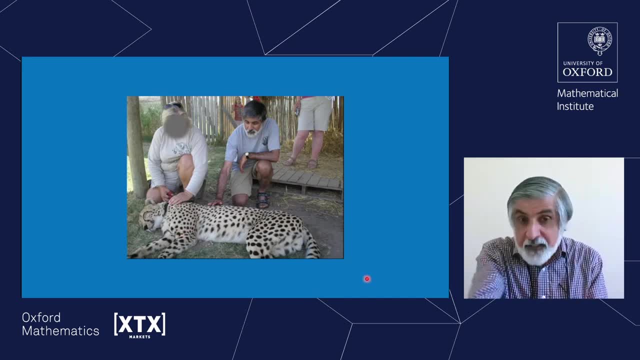 cheetah and it's sleeping Okay, so I didn't do anything bad to it. It's just having a nap and I'm just stroking it. And this is what we mean by pattern. See all these spots. Those are patterns. 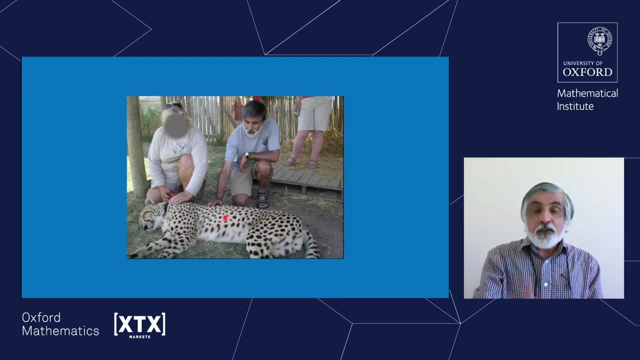 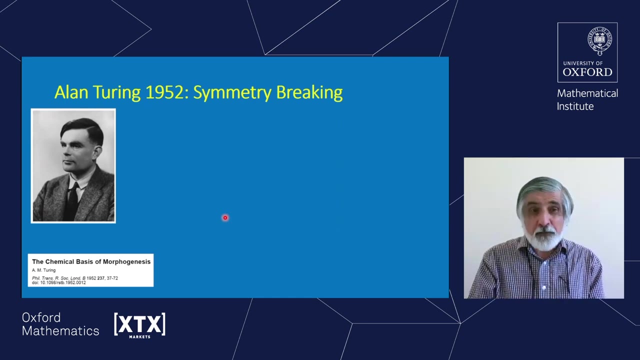 Stripy tail. Here's another pattern: Digits, Five digits, Pattern of boulders. Question is: how do these patterns arise? So I mentioned at the beginning of the talk Alan Turing. he starts to look at this problem in the early 1950s. 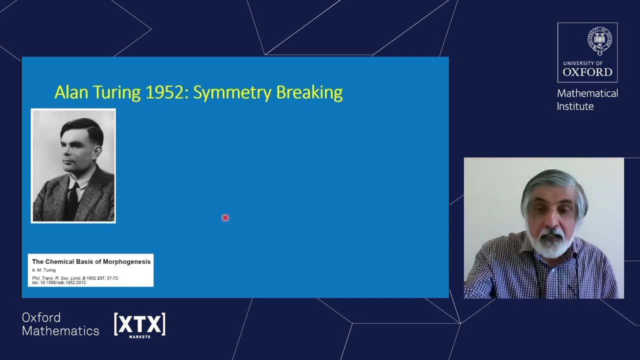 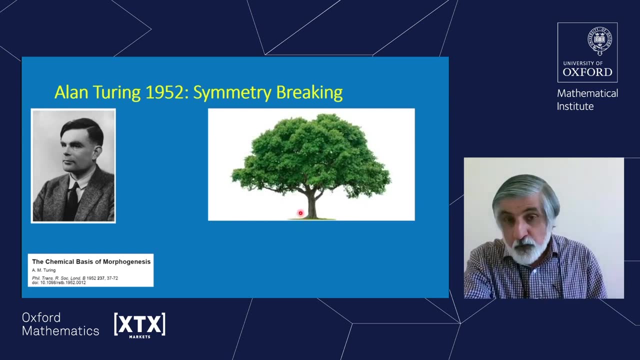 before he tragically died. So he had this notion here. Think of this tree, and the tree is growing. And suppose you were to look at this tree at this point here. What you would see if you looked down on it would be a circle. 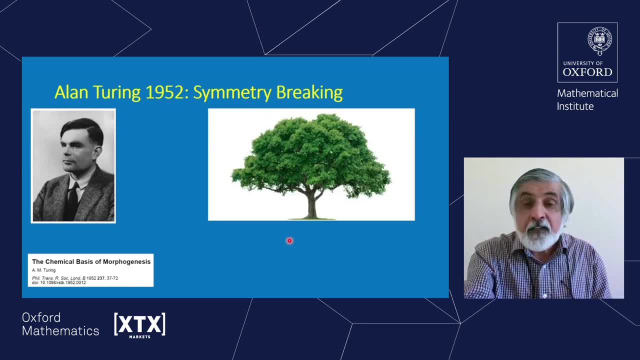 And the tree is growing, And then at some point here that circular symmetry is broken by this branch. So Turing had the following idea: There must be some growth hormone that's causing this to grow, And then it's, and so if the growth is symmetric, 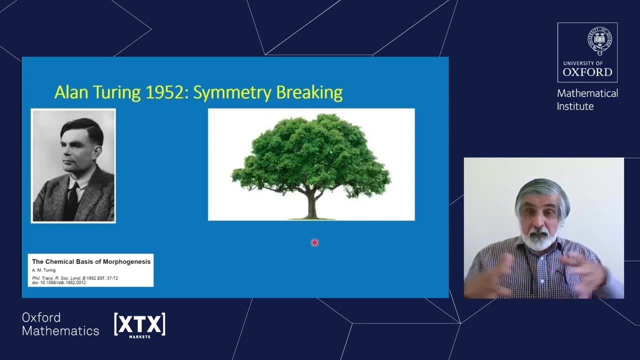 that growth hormone must be symmetrically positioned, Then at some point that symmetry must break, must become destabilized, And then you have a asymmetric growth profile, asymmetric concentration profile of the growth hormone, and that leads to an asymmetry in the growth. 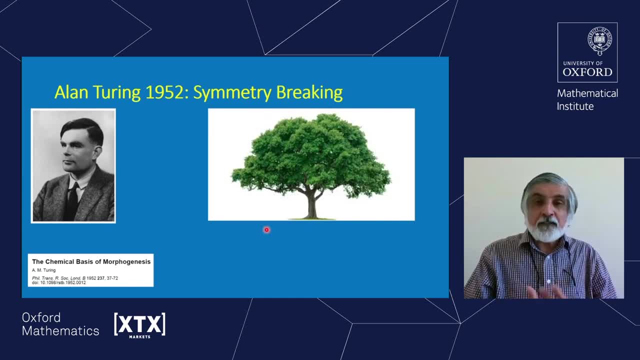 So you can think about taking this even further And you could say that, instead of that asymmetry in the chemical resulting in an asymmetry in growth, it could result in an asymmetry in fate determination. So, for example, where the chemical concentration is high, 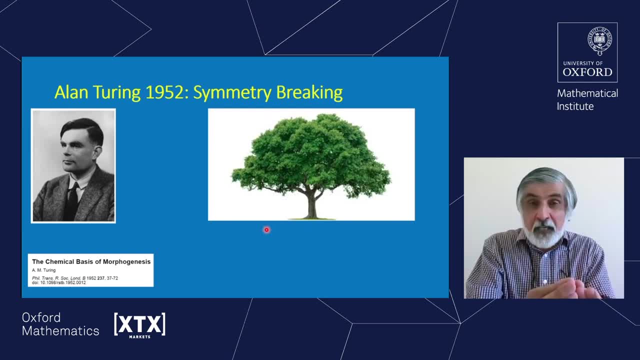 that could result in cells adopting a certain type of fate. Where the chemical concentration is low, the cells do something different. So they form bone if the chemical concentration is high. They don't form bone if the chemical concentration is low. And he called these chemicals. 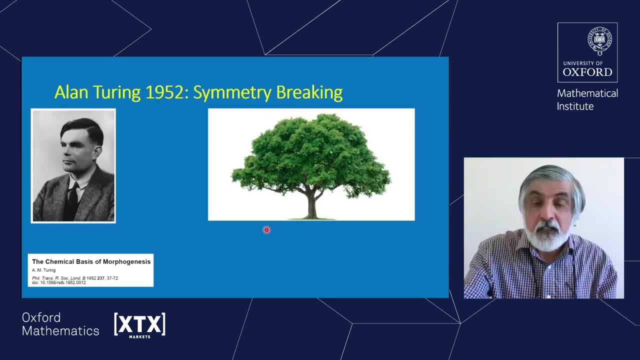 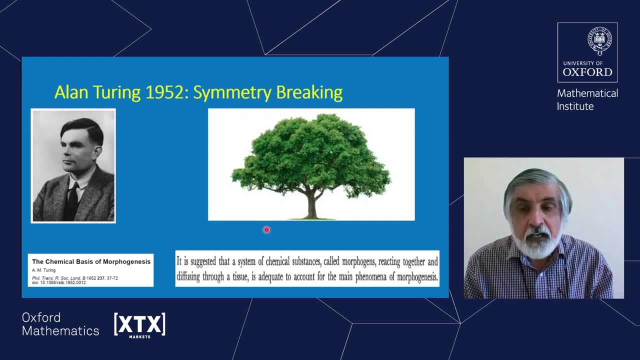 morphogens, And that's what he said. It is suggested that a system of chemicals called morphogens reacting together and diffusing through tissue is adequate to account for the main phenomena of morphogenesis, meaning pattern formation. And in fact, many, many years later. 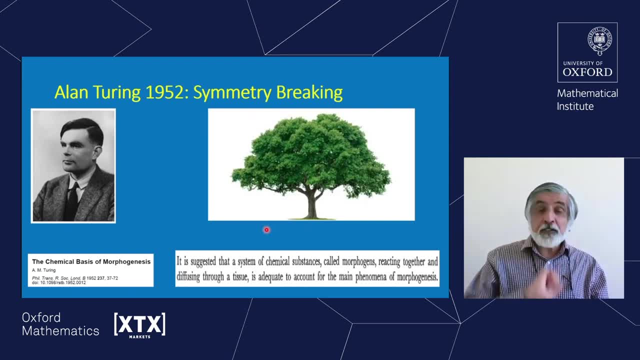 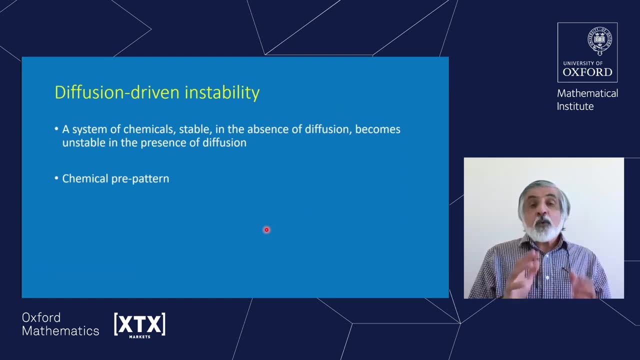 people have actually found morphogens. These were predicted by Alan Turing 30 years before they were found. So the question is: how do you get this symmetry breaking or instability to arise? And what Turing said was: diffusion caused the instability. Now this seems really counterintuitive. 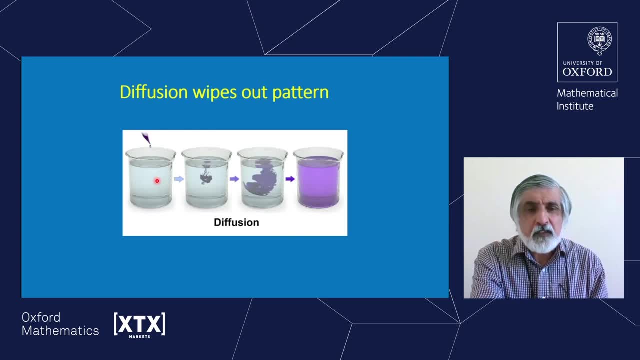 because think, suppose you start off here, here's some water, and you put a blob of ink into the water, so you have a pattern here, Ink here, nothing else here. Come back a little while later the pattern's disappeared. 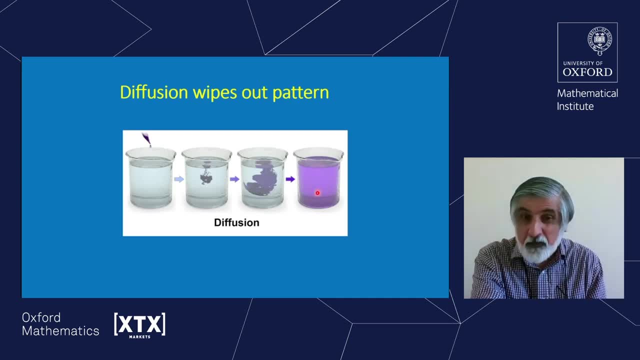 There's no spatial structure here, it's all the same. That's because of diffusion. The random movement of the molecules around has ended up meaning they distribute uniformly, And yet Turing was saying that diffusion causes pattern. That seems really counterintuitive. 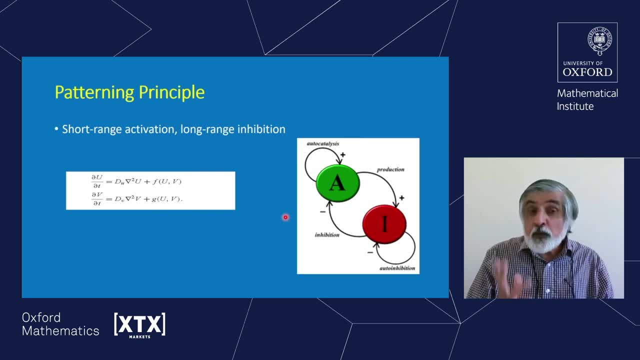 So he wrote down a system of two equations, two chemicals, U and V, and there's the diffusion term, here and here's the reaction terms. And what he said was: for this to happen, you need a number of key things. You need one chemical to produce. 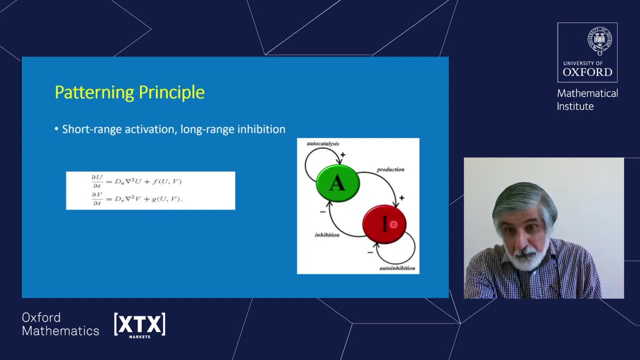 to produce the other chemical and to produce itself, and then this chemical inhibits this chemical. So this one he called the activator, because it activates the inhibitor and the inhibitor inhibits the activator. So let's think about this. 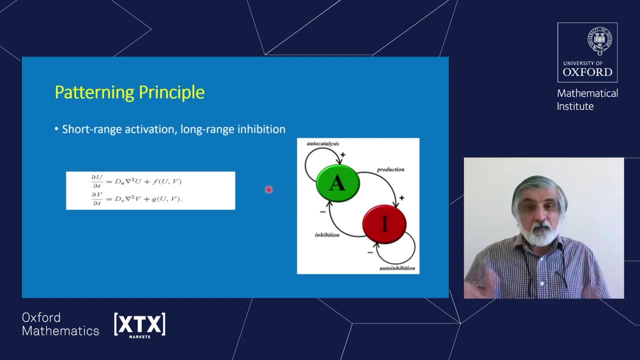 Suppose you've got a pile of an activator. it's catalyzed in itself, so it's producing more of itself, but it's also producing the inhibitor. Then the inhibitor inhibits the activator. So if there's more activator, 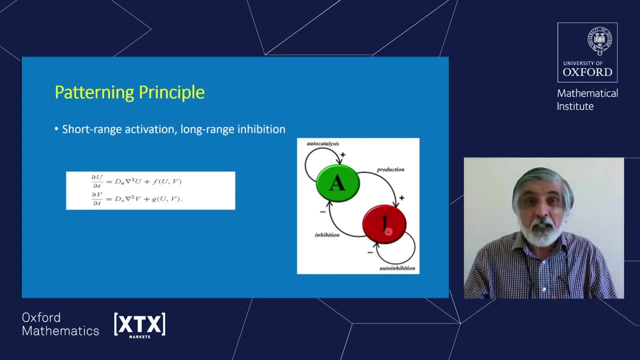 there's more inhibitor and that pulls the activator down. So you can imagine getting to an equilibrium where you've got a level of activator and a level of inhibitor and that's stable, because if you added more and more of it. 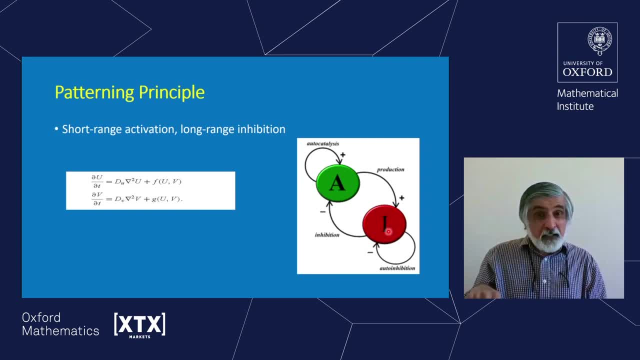 more activator. that would activate the inhibitor, which would make more inhibitor, which would pull the activator back down. There's less activator, there's less inhibitor. the inhibitor will come back down and you get back to the steady state. 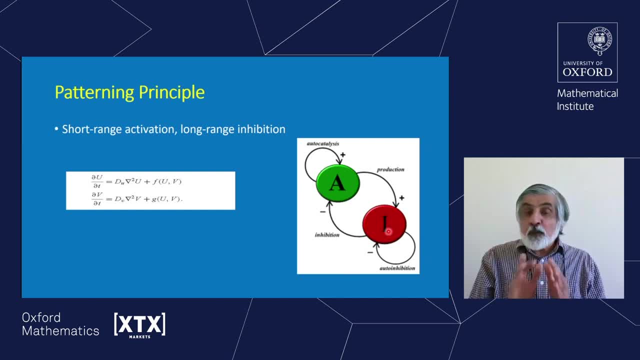 So this is stable. But now suppose we have diffusion and suppose that the inhibitor diffuses faster than the activator, Then what will happen? if you do that perturbation again? the activator starts to produce itself, starts to grow, produces the inhibitor. 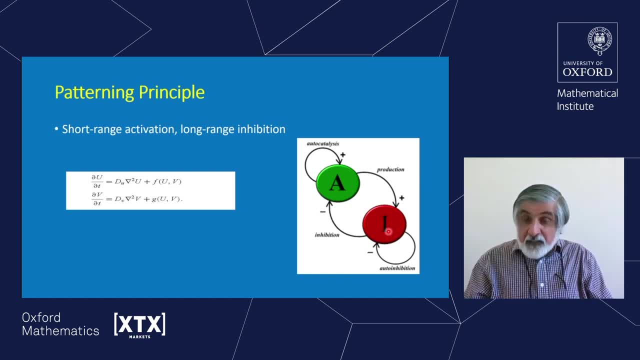 Now the inhibitor. some of it inhibits the activator, but a lot of it gets out of the way. So there's not enough inhibitor to inhibit the activator. So now the activator grows even more, Produces more inhibitor. it goes away. 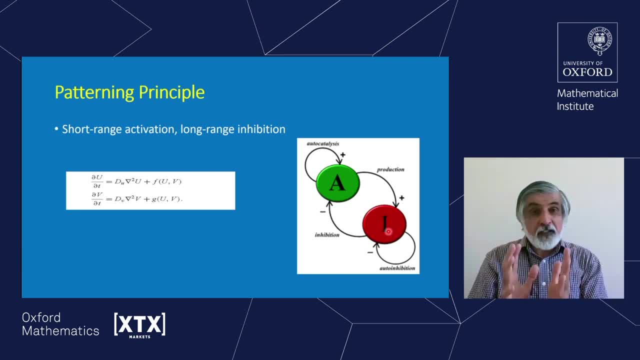 So what you'll end up getting will be lots of activator surrounded by lots of inhibitor, a spatial pattern. So our intuition that diffusion gets rid of pattern is based on one thing: diffusing- And that's the singular case- As soon as you have. 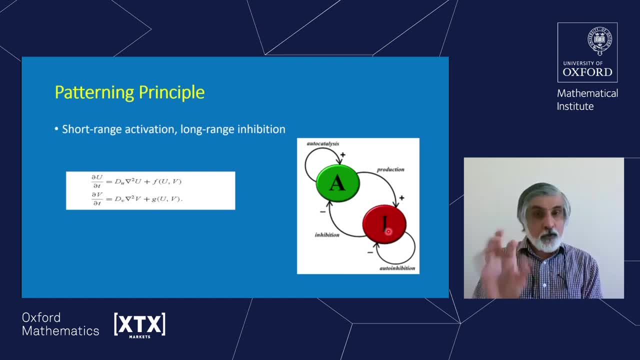 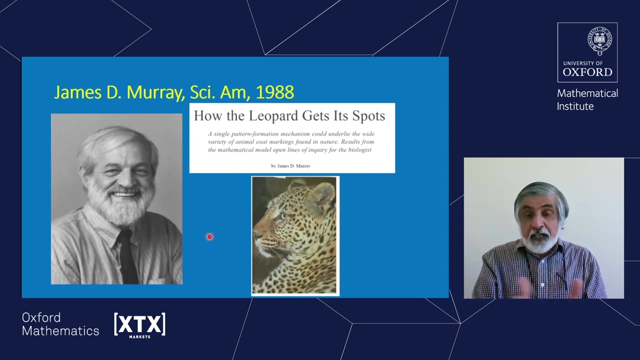 more than one species. chemical diffusing diffusion can drive pattern. So this is a nice example of mathematics: pointing out where our intuition is wrong and building our intuition. And Turing used mathematical analysis to prove this And this, this idea of reaction diffusion. 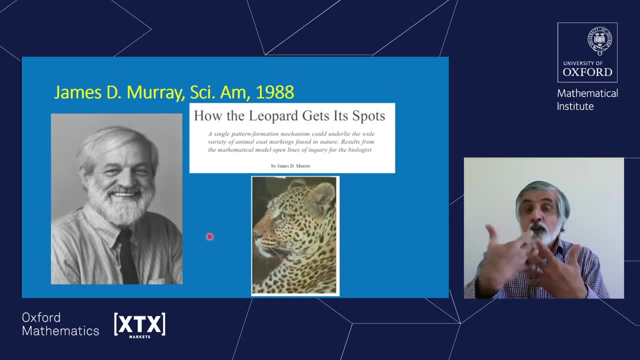 forming a pre-pattern for animal coat, markings, patterns and various other things has been used a lot, And so Jim Murray, who was my supervisor when I was a graduate student here in Oxford. very famous paper of his here where he shows how you can get patterns. 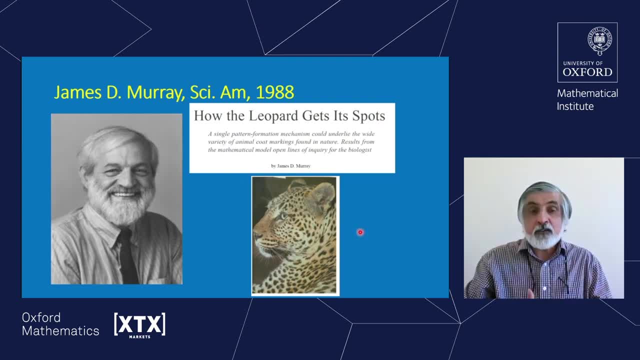 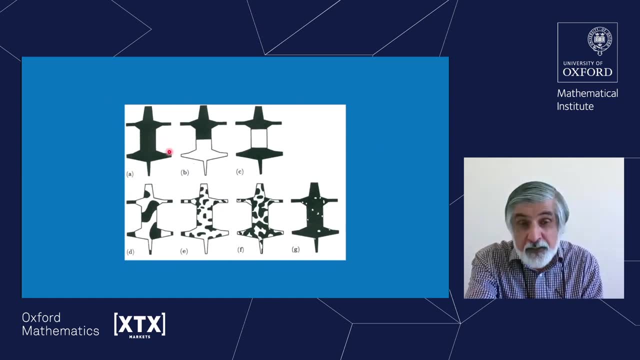 that look like the spots on the leopard, and you can get those by a reaction diffusion system. And here's another idea, idea here. So this obviously looks like an animal coat marking And what's happening here so you can think about here. 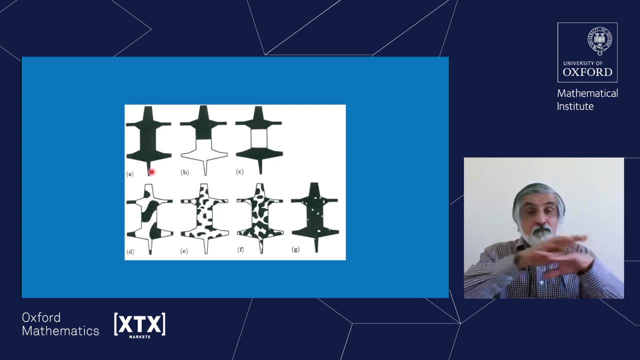 there's no pattern. The chemical doesn't form any pattern. And then, as you move here, the domain has got bigger. but he scaled the domain back so it fits on the graph on the piece of paper, Otherwise the pictures would get too big. 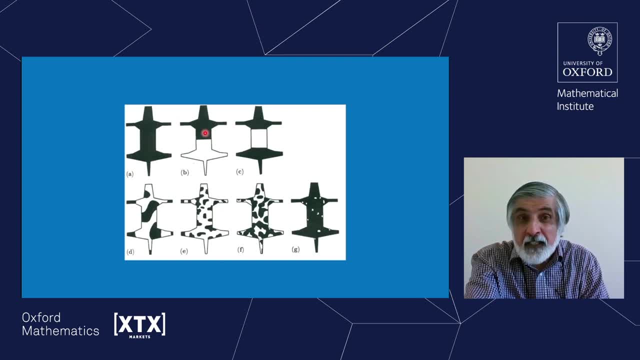 But this is for a larger domain And now you start getting some pattern. As you increase the domain further, you get more pattern. Further you get more, you get more, you get more. So the way you can sort of think about these, 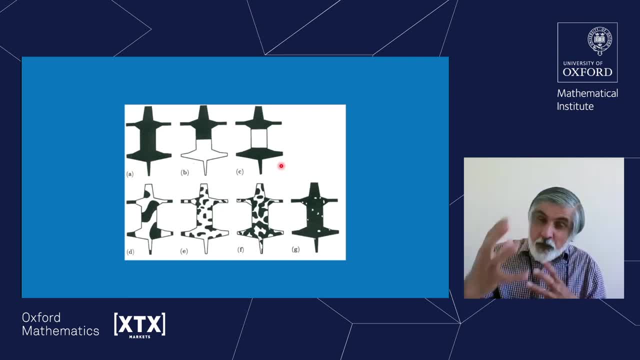 is that basically these patterns it turns out if you look at them, they're what are called eigenfunctions of the Laplacian And on these sorts of diagrams here they're essentially mixtures of sines and cosines And what you can think as 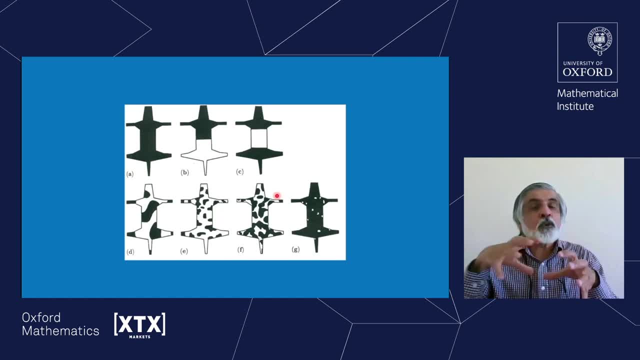 as the domain gets larger, you can fit more sines and cosines in and get more complicated patterns. So therefore, the prediction is that there should be an animal that looks like this and an animal that looks like this. Now you might have seen an animal. 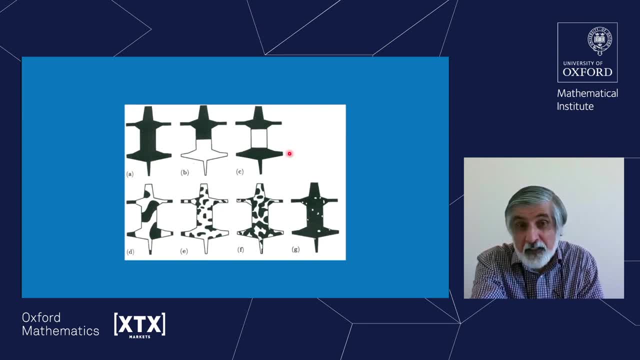 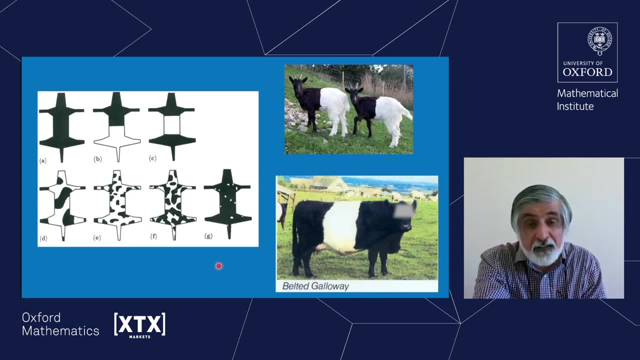 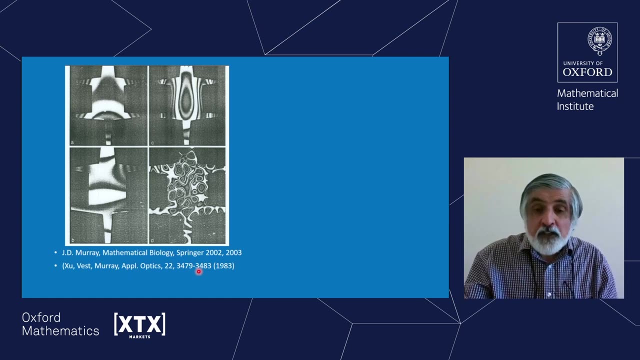 that looks like this. maybe not seen an animal that looks like this. Well, here we are. These are not photoshopped. This is Valley Goat. This is Belted Down. So, as I mentioned these eigenfunctions of the Laplacian, 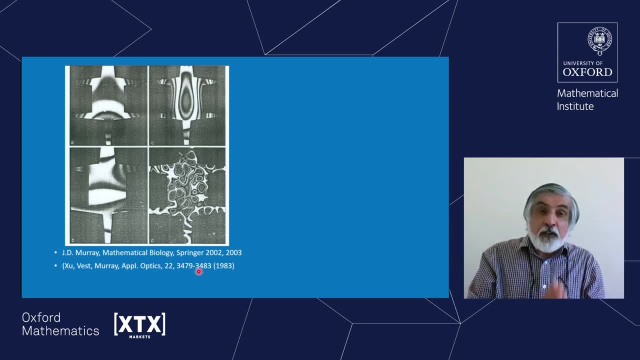 form the pattern. So are there other places in mathematics or in science where we see eigenfunctions of the Laplacian. Well, if you vibrate a plate or a drum or strum a guitar, the vibrating modes are eigenfunctions of the Laplacian. 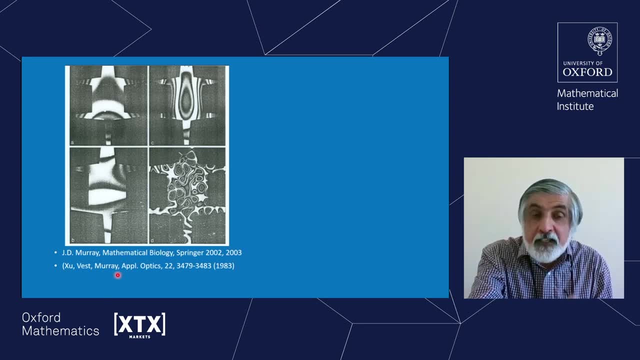 So these authors here had the idea that if you vibrated a plate that looked like an animal coat marking and you could visualize the vibration, then, since the vibration are eigenfunctions of the Laplacian and they're proposing that animal coat markings are eigenfunctions of the Laplacian, 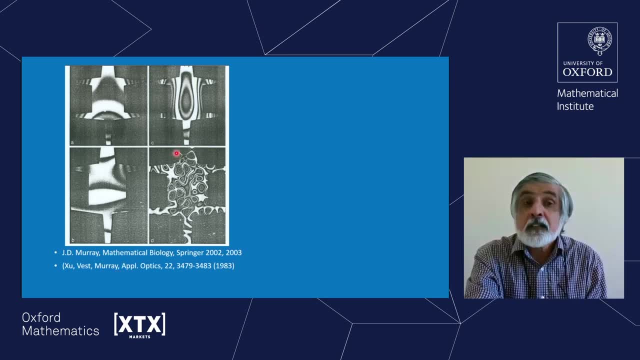 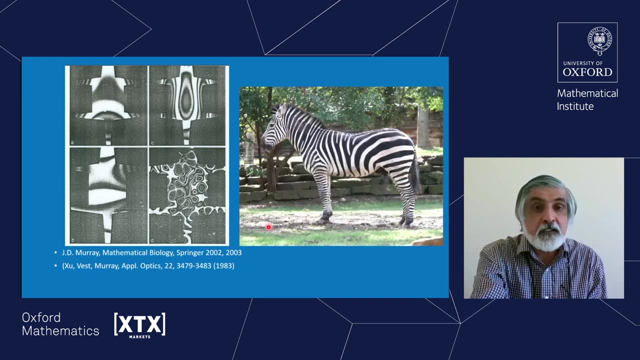 then you should see animal coat markings. So this is the vibrating plate And look, These are very like animal coat markings. I mean, look at here, You got that sort of thing here. Here's a zebra, That sort of thing. 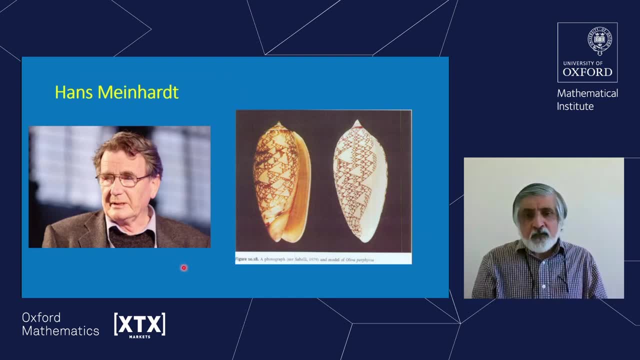 And Hans Meinhardt, and this is taken from his book The Algorithmic Beauty of Seashells, a beautiful book, where this is a real seashell and this is a pattern of seashell generated by system of reaction-fusion equations. 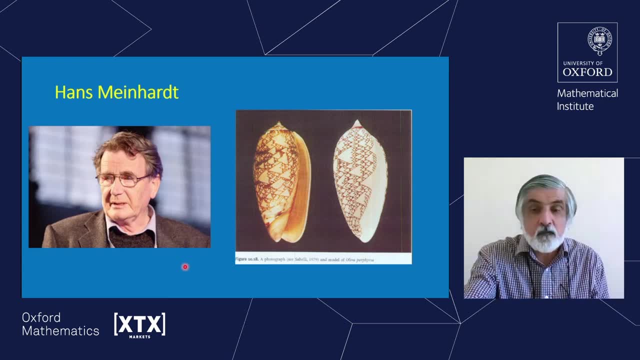 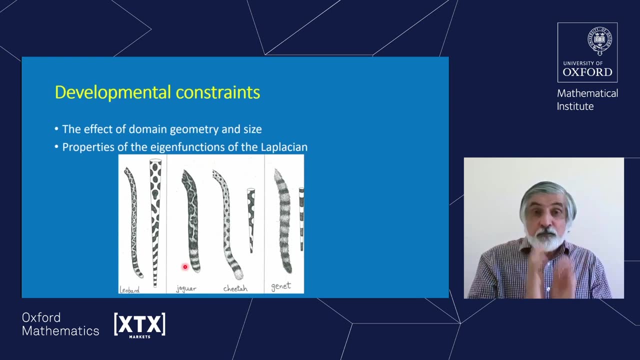 And the book is full of beautiful pictures like this. So the eigenfunctions of the Laplacian have certain properties. One of their properties is that as the domain, the geometry changes, the pattern changes, In particular as the domain becomes narrower. 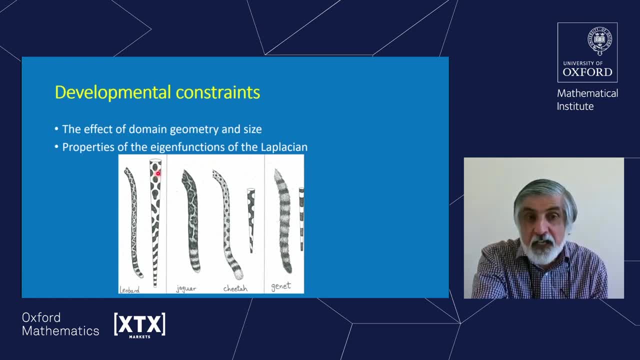 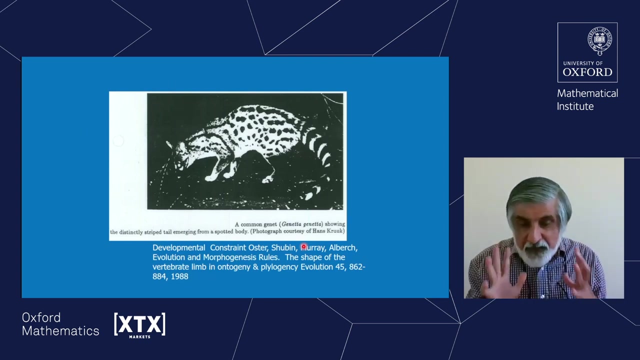 and more one-dimensional. the pattern changes from being intrinsically two-dimensional, like spots, to becoming one-dimensional, like stripes. So here is the model and here is an animal Model- animal. So, if we take this a bit further, what this tells us. 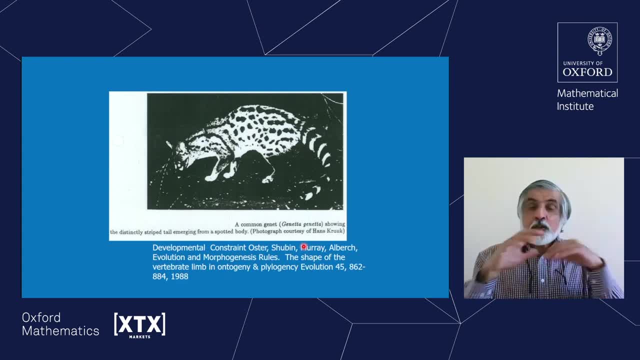 is that if you have a domain and you see a pattern on it and if the only thing you change is the domain geometry- so, for example, you go from a fat big domain to a small domain- then the pattern cannot get more complicated, because the complication of the pattern 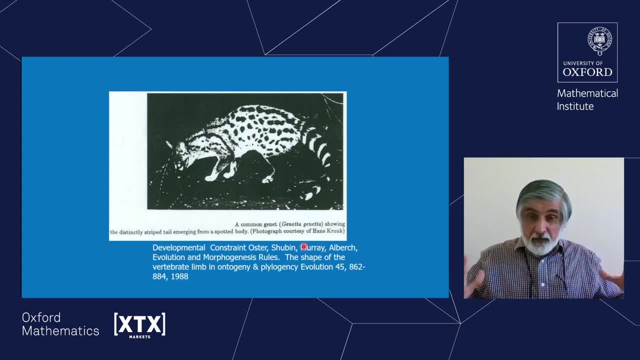 increases with domain size. So if you have an animal that's got spots on its body and then you look at the tail, which has got a narrower, more one-dimensional geometry, you will either see spots or stripes- more likely stripes. On the other hand, if on the animal body you see stripes, then as you narrow the domain you will either see stripes or no pattern. You will not see spots because that would mean the pattern getting more complicated. This is the idea of developmental constraints, And this is a paper. 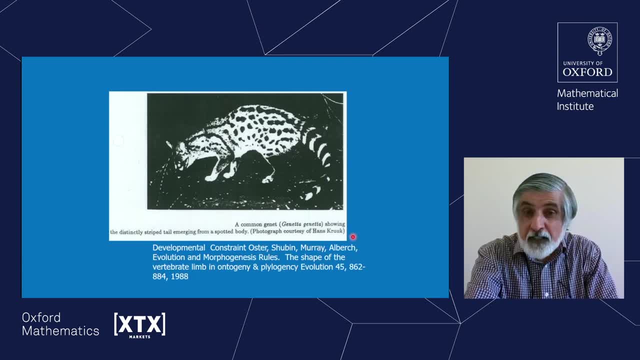 where two theoreticians, Foster and Murray, came up with this idea from the mathematics, And these are two biologists who came up with the idea from actually looking at skeletons, looking at coat markings, etc. So these were data driven, these were mechanistically driven. 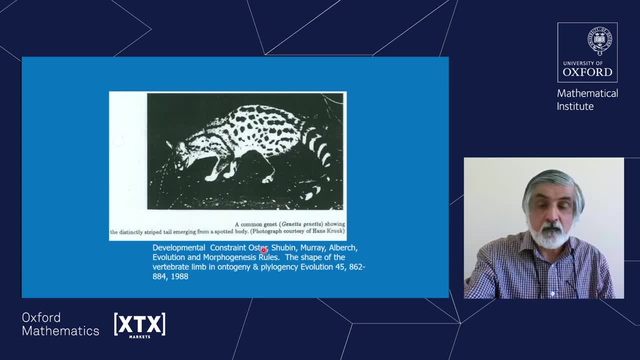 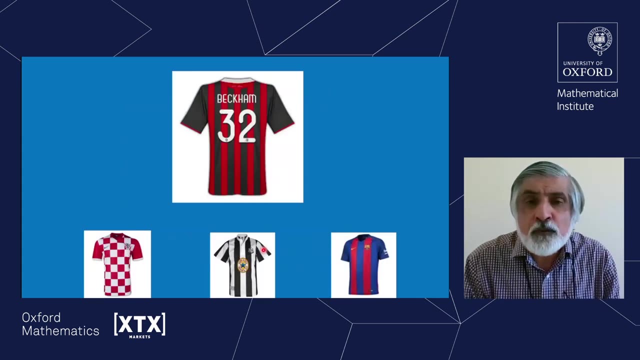 These are mechanistically driven results. So the idea is that a spotted animal can have a stripy tail, but a striped animal cannot have a spotted tail. Okay, So now let's move to Premier League football shirts. or football shirts, they're not Premier League. 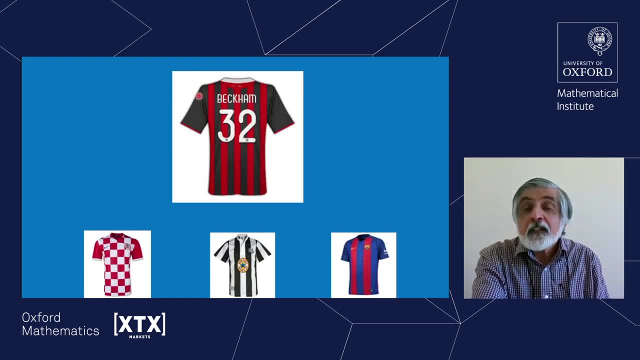 Here: stripy body and simpler pattern on the arms. Spots, simple pattern, Stripes, stripes, stripes, no pattern. So these obey Turing's model. The pattern on the sleeves is not more complicated than the pattern on the body. 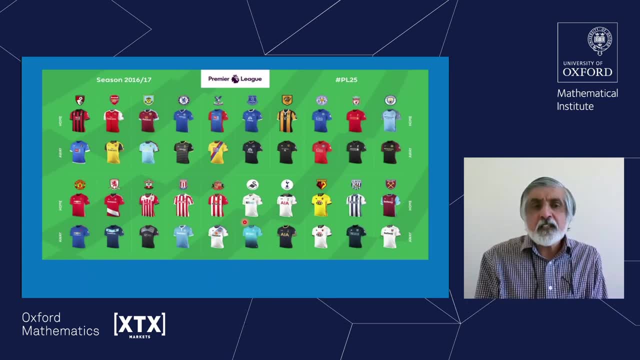 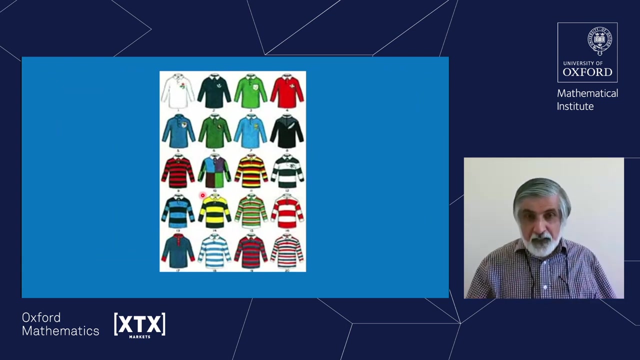 Here- these are from 2016-2017, the Premier League, and virtually all of these satisfy Turing's theory. The pattern on the sleeves is not more complicated than the pattern on the body. Rugby shirts: same thing Pattern on the body. 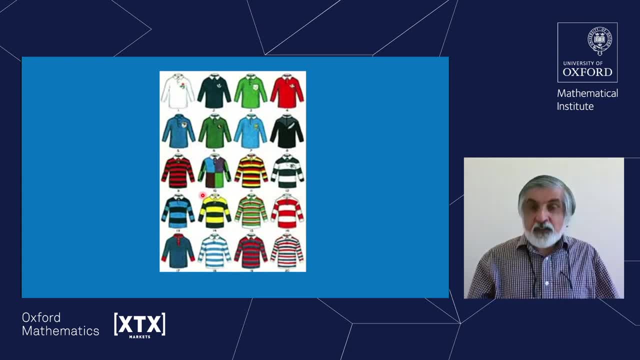 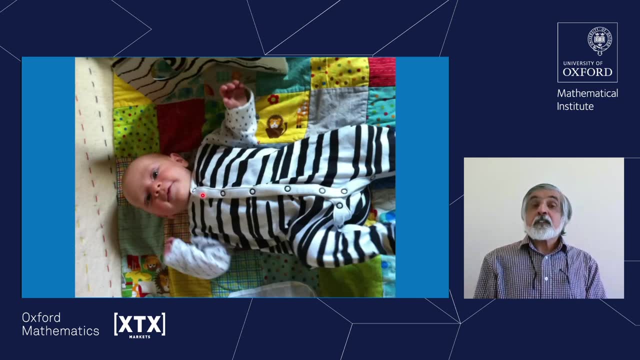 is as complicated or more complicated than pattern on the sleeves, But there are counterexamples. This is the daughter of a former graduate student of mine and he sent me this photograph and instead of saying: look, how beautiful is my daughter. 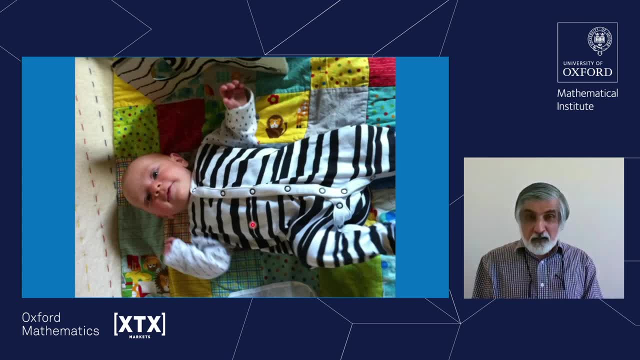 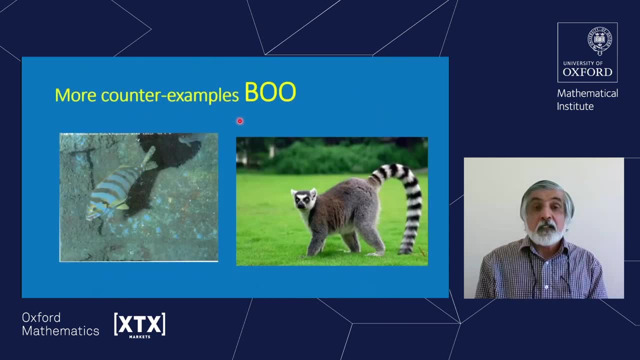 he said: look, contradiction to Turing's model: Stripy body, spotted arms. Here are some counterexamples. So when you see these animals, you should boo at them because they don't satisfy Turing's theory. Stripy body. 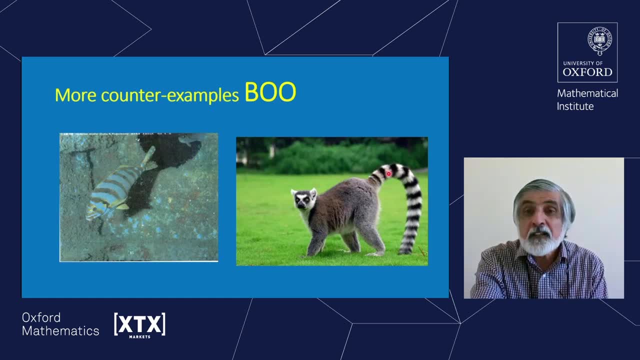 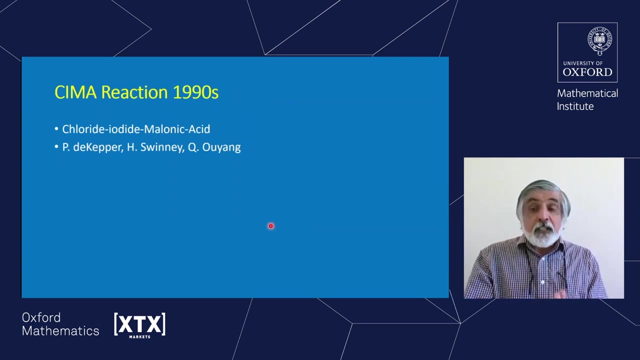 spotted tail, No pattern pattern. These are counterexamples. So what you would think is going on here is that not only is the domain geometry changing, but something else is changing. Now the question is: do these occur in nature? 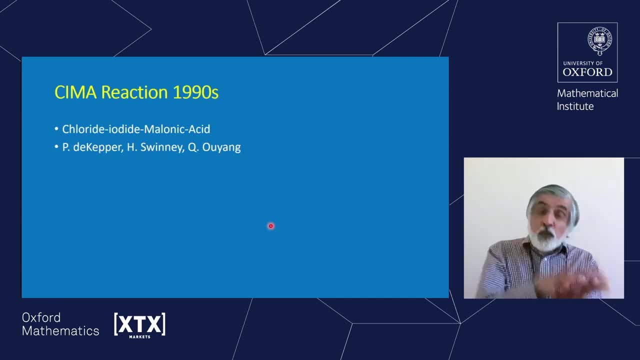 in the actual biological system. We know that morphogens occur. There's still a huge controversy as to do these patterns occur because of the way Turing said reaction to fusion. They've been shown to occur in chemistry, So in chemistry these are Turing patterns. 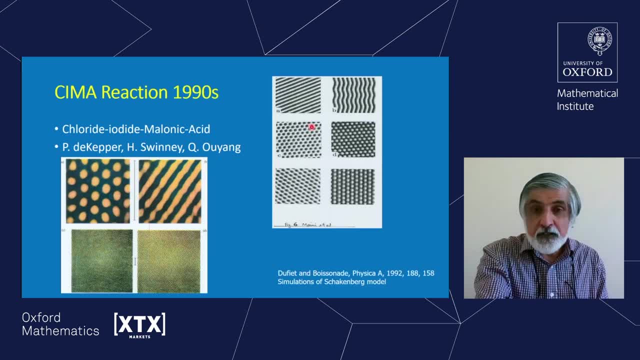 They've been found in chemistry. So in chemistry, and here is the simulation- This is actually just taken from this paper- showing that the model predicts you can get these types of patterns like this. You can get spot hexagonal patterns. 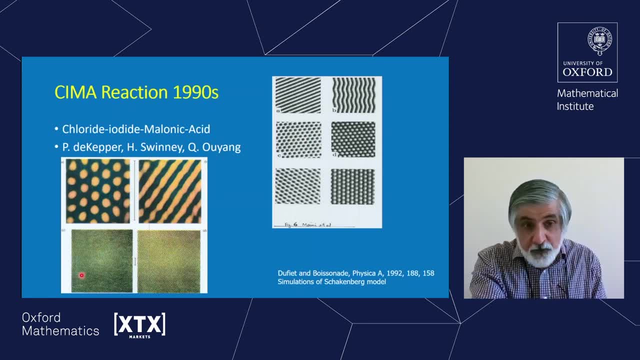 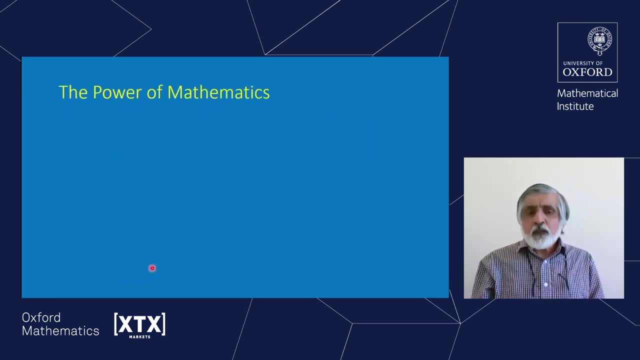 like this. In fact, I haven't got the picture here, but you can also get these labyrinthine patterns. So hopefully what I've shown here is that by understanding the mathematics in one area of biology or chemistry or mechanics, you can understand. 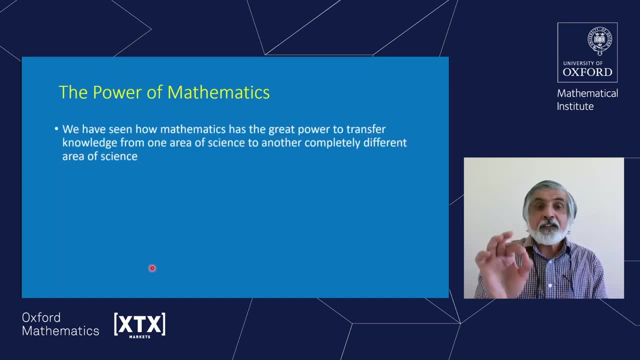 other areas of science. And that is the power of mathematics, Because by abstracting, by the art of modeling, which means you abstract processes, many different processes have fundamentally the same principles. So you could argue that mathematics is what unifies science. 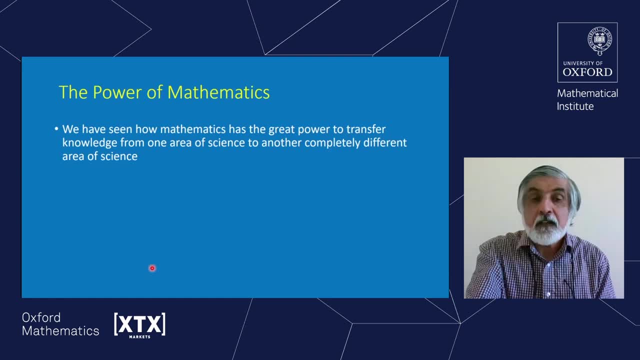 by bringing out these processes that are common across different areas, So they can transfer knowledge from one area to science to another area of science. It shows that mathematics is really powerful. But remember, with great power comes great responsibility And you have to be careful. 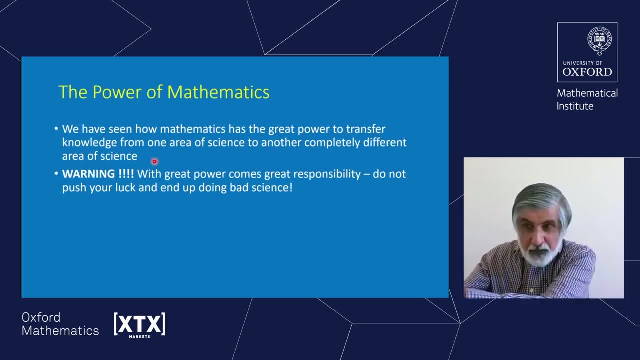 not to push your luck, not to look at something, some scientific phenomenon, and say, oh, that pattern or that structure looks like this other area of science. So if I understand that area of science, I understand that area. That is bad science.